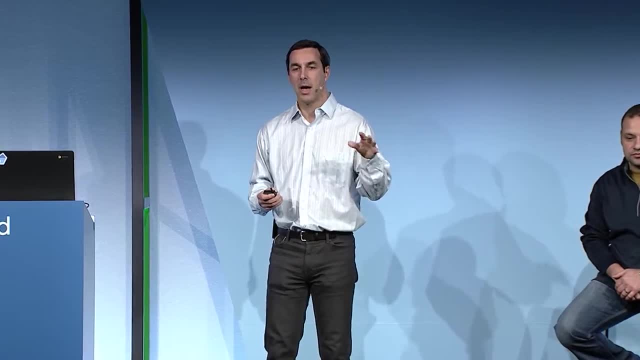 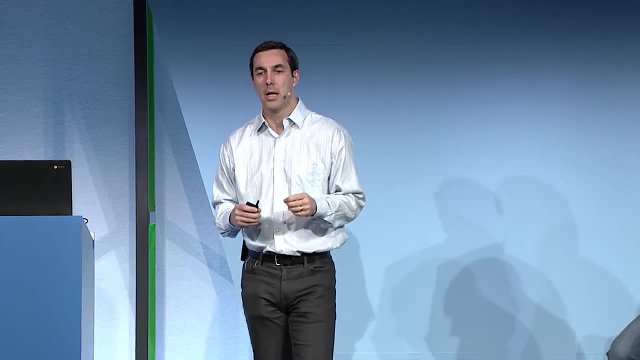 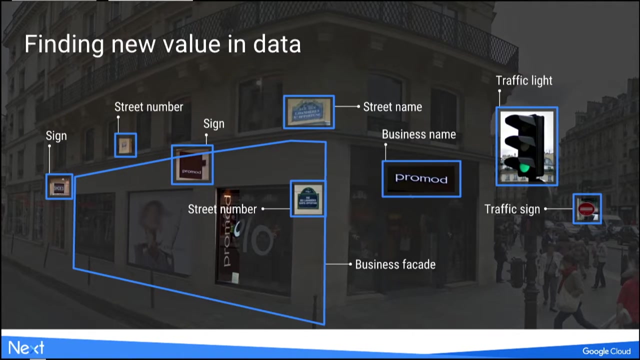 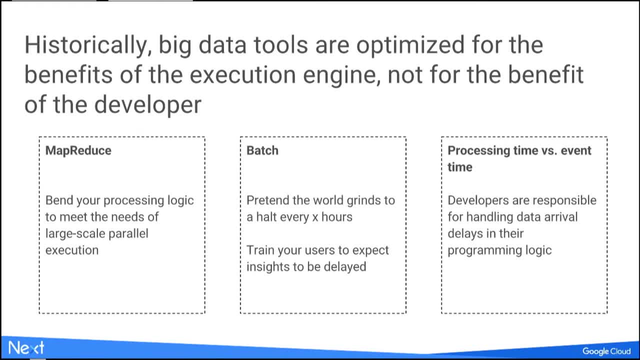 But really MapReduce forces the developer to learn a new way of thinking And especially if they have more complex pipeline they have to optimize. It's actually a lot of work to write really good MapReduce, But it's very easy then, once you've done it in MapReduce for the infrastructure to parallelize your work. 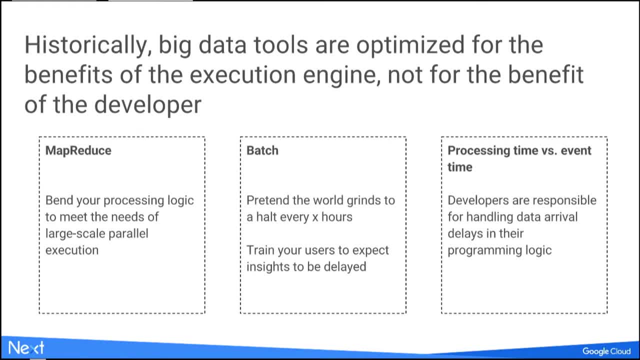 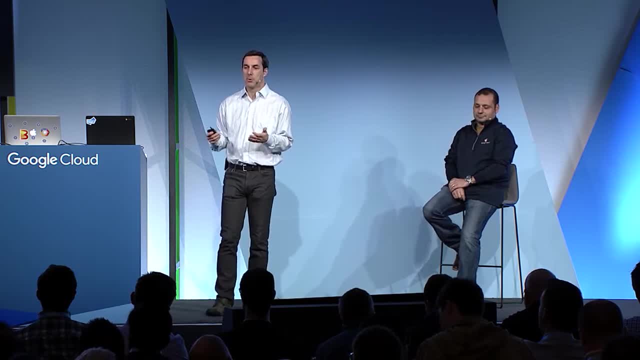 And so that was the tradeoff. But that has limited access to big data to a much smaller subset of developers, And that really doesn't have to be anymore. Same thing with Batch. Same thing with Batch. For some reason, as an industry, we tend to assume that there's something natural about Batch. 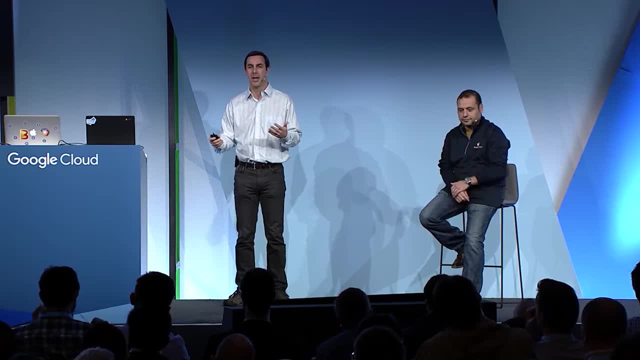 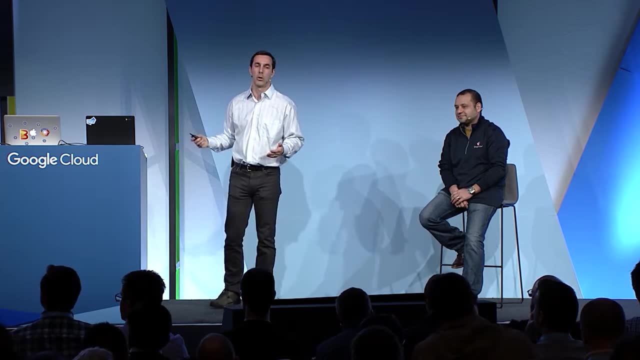 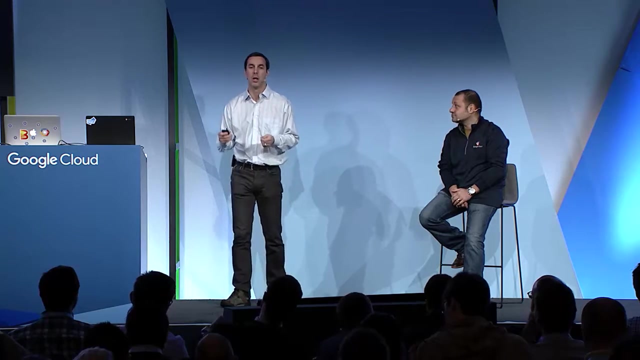 That, of course, things at scale happen in Batch, And in reality there's really nothing intuitive about that. It's just the force of habit that makes us think about Batch. The world doesn't work in Batch. Things happen continuously, And so the tools have been forcing us to think in Batch mode when really we shouldn't. 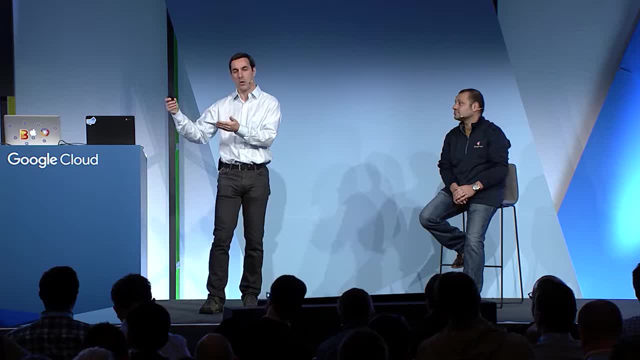 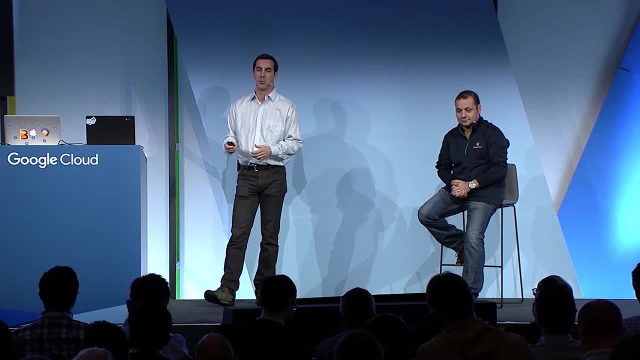 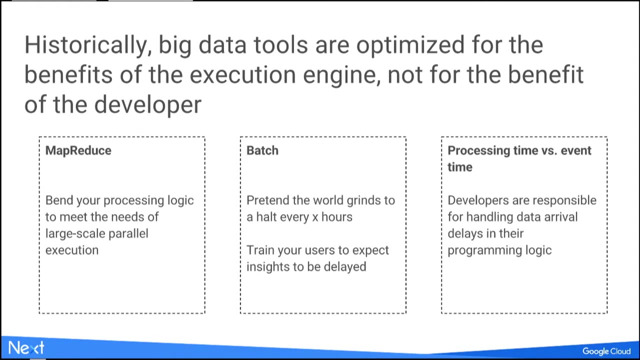 Also, they've been forcing us to think about object in terms of events, in terms of when they're processed, when they arrive In your processing logic, as opposed to when they actually happened, which is not always the same, And so the reason why right now there's a lot more easy access to big data is because those constraints have really been removed by a much more mature programming model. 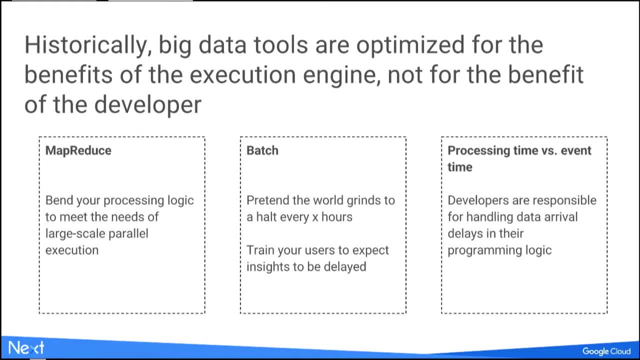 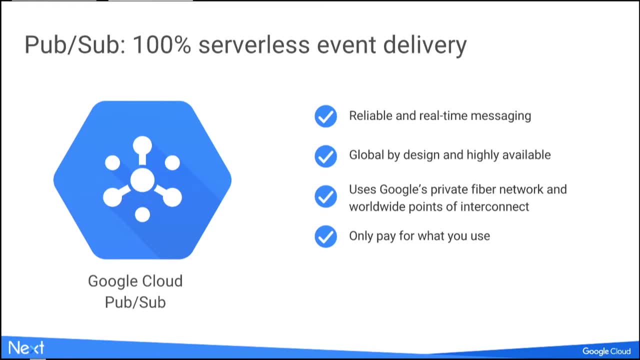 And Reza is going to tell us about that. Thank you very much. So it's been the last couple of years. I think I've been very, very lucky in that I've actually worked directly with our customers doing a little bit of that. 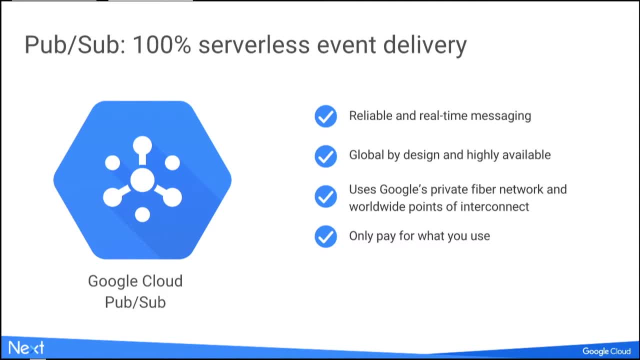 That code stuff to actually convert batch processing pipelines over to streaming. And actually, before we talk about data flow itself, let's think about how we're going to collect this data. So let's just take two simple examples of stream data. One is IoT data. 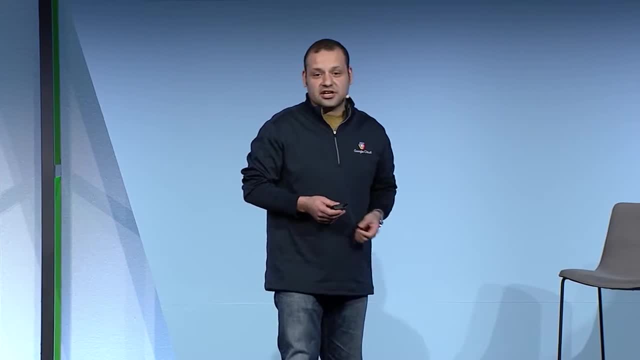 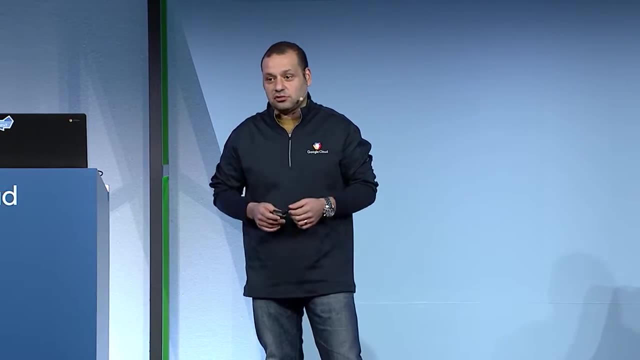 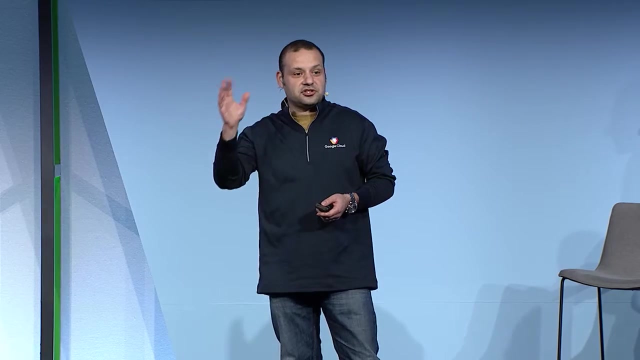 Imagine there's lots of factories that we have. There is IoT devices: measuring temperature, measuring number of machines are on. All of these devices are sending information to somewhere, And the other use case that commonly come across is clickstream. So as users are clicking around your applications on a website, they're doing stuff on their mobile. all of these events are clickstream information that's being recorded and being processed. 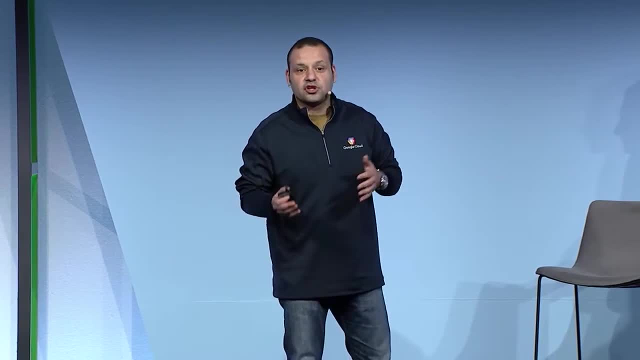 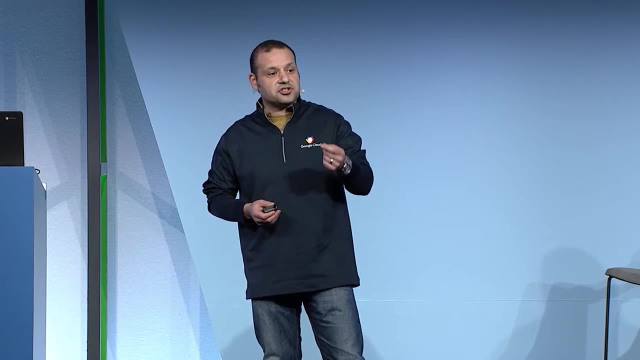 Now, normally, obviously, that usually gets processed by batch processing, But as we move to stream processing, we now need a way of capturing that, And Google Cloud PubSub API is a publish and subscribe API. There's no running up machines. 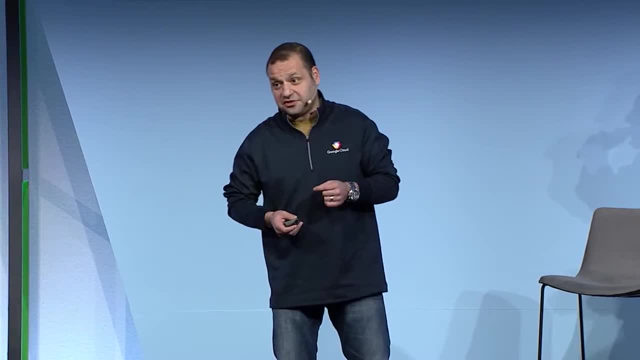 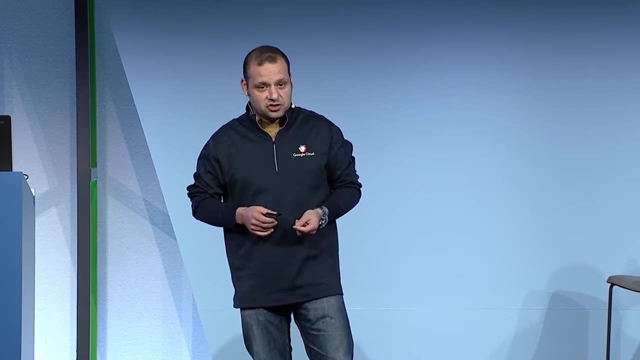 It's fully managed service. I essentially- and it's the easiest part of any POC that I do with customers. it's four or five clicks. I get a topic created And what that allows you to do is, from anywhere in the globe, you can send information to it. 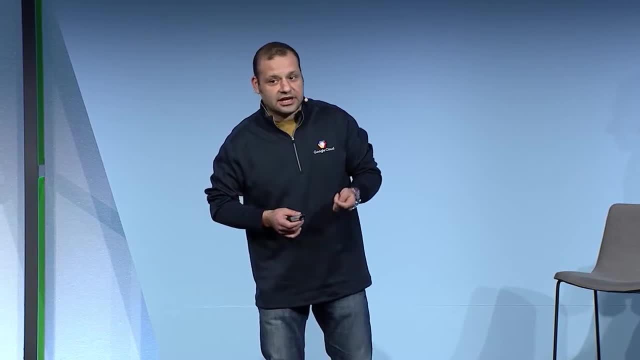 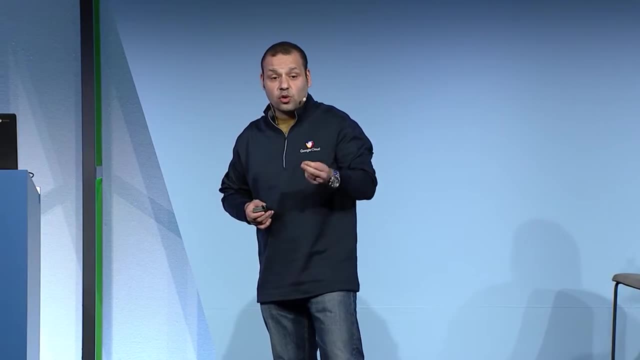 We can process it in any region that we like. It is highly available And it means that when a message is recorded and acknowledged by PubSub, it will actually keep it in the system for up to seven days or until the subscription pulls that message and acknowledges that it's been processed. 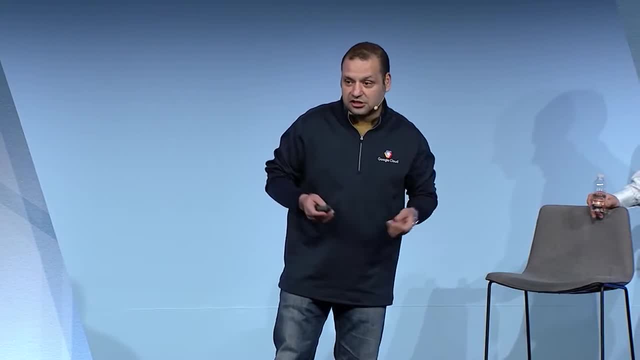 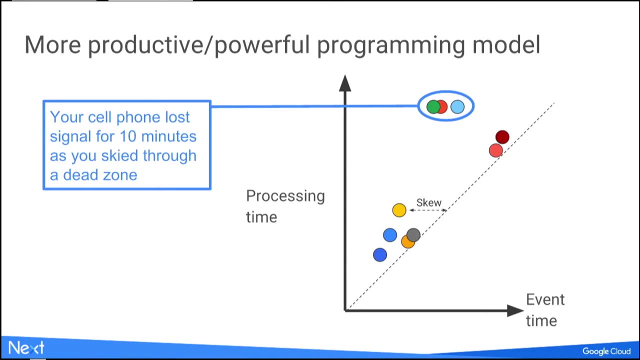 So this piece usually takes a few minutes to set up in any POC And it will deal with several messages, a second or, as with some of my customers, hundreds of thousands of messages per second. So going on to Dataflow itself, historically it's been considered that if you wanted accurate processing you tended to need a batch processing pipeline. 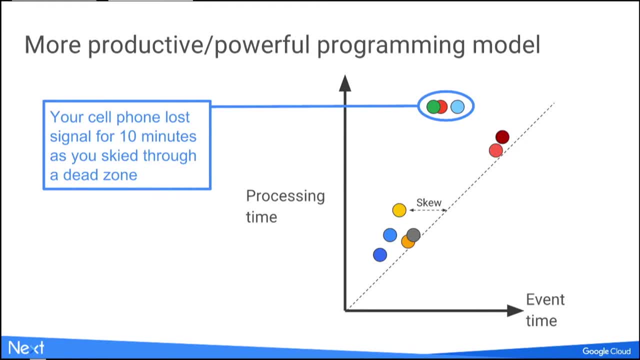 So you would have batch technology. You would collect all the files at the end of the day, maybe do some corrections, some ETL, and then do some batch processing on it. If you wanted low latency, you would then go and build a completely separate technology stack that would absorb these streams of data and do some processing for real-time dashboards, et cetera. 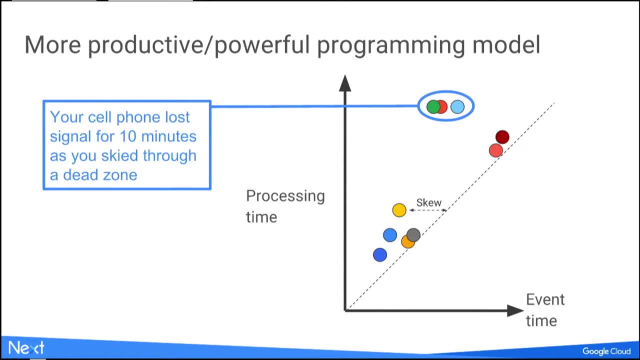 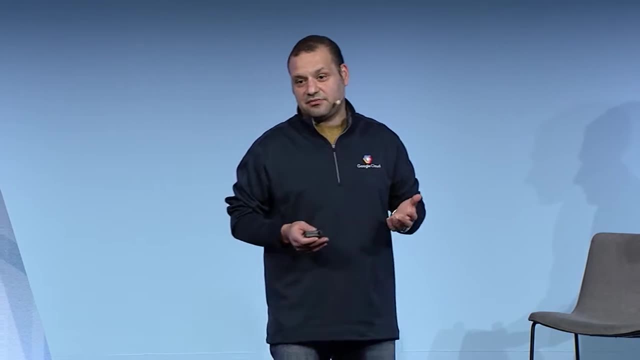 But it was always considered that that was the best way to do it. It was not accurate enough for something like a billing pipeline. Now why is streaming difficult? Well, let's take that simple example of clickstream Now data. one of the common problems with streaming pipelines is late data. 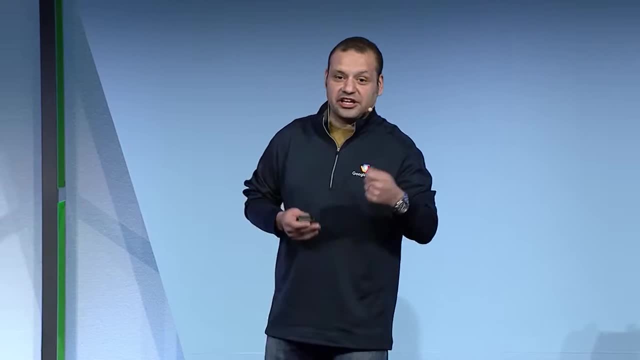 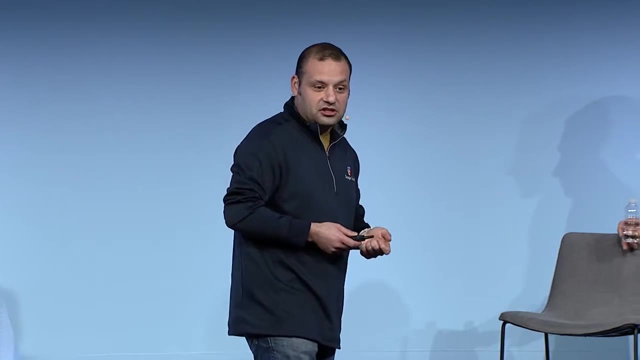 So imagine one of your applications is a mobile device. Your users are going to be going in and out of cell range. They're going to lose connectivity. They're still using, potentially, the application As it's recording information when it suddenly comes back online. 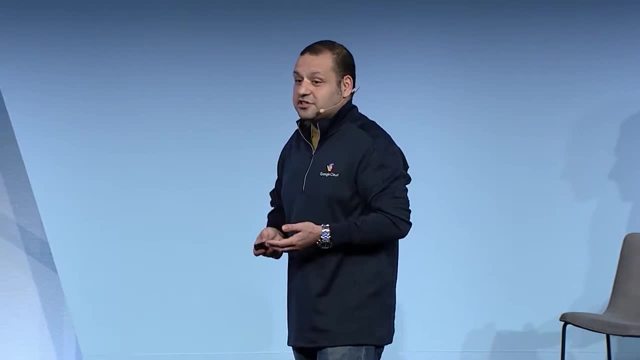 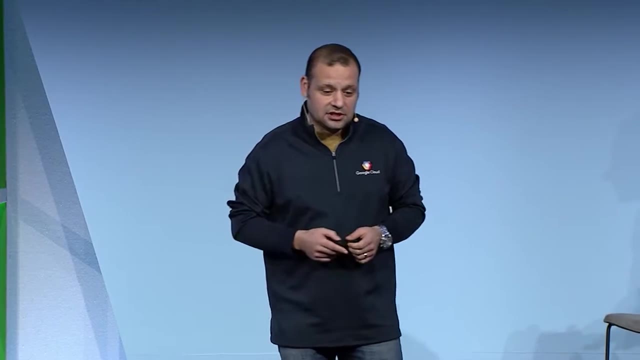 it's going to send a clump of data. Now, if one of the things that we want to do is accurately count how many people are on our applications at any point of the day, at this point we've got a problem because we're going to miscount. 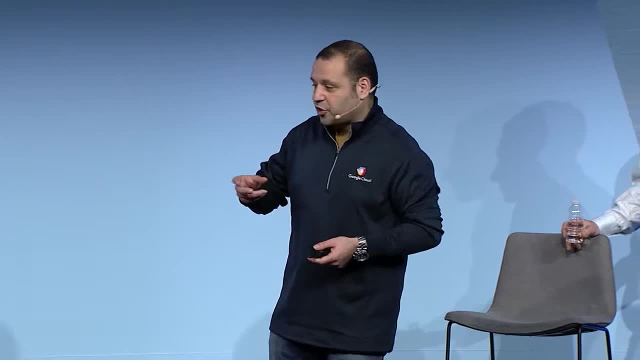 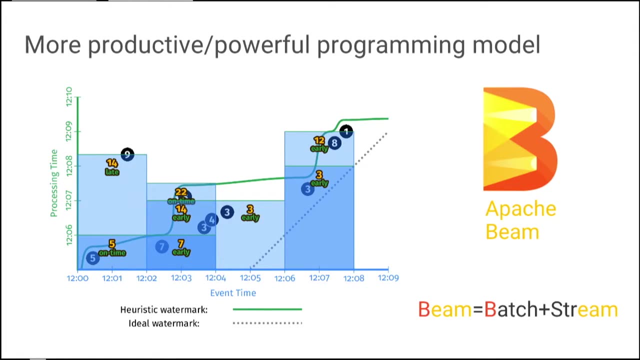 And what Dataflow allows us to do is. it gives us a powerful programming model that is geared towards streaming. It can deal with batch as well, But what it allows you to do is deal with things like late data. It gives you simple primitives to deal with things like windowing and sessionization. 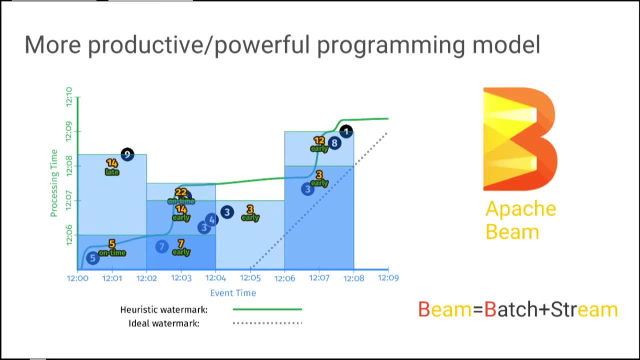 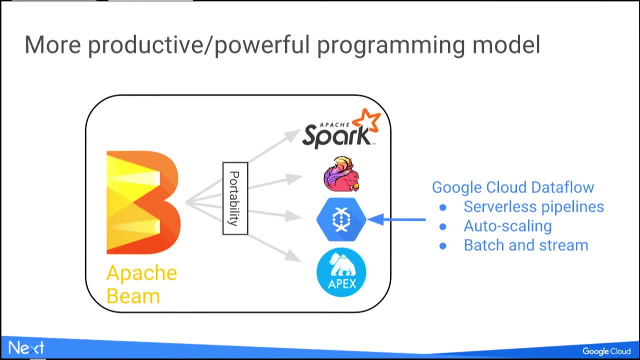 And the Dataflow programming model allows us to do that. The Dataflow programming model and SDK was contributed to Apache Beam. It's now an open-source project And Apache Beam- there are several folks building runners for it, So we have Spark and also other execution engines like Flink and Apex who are building runners. 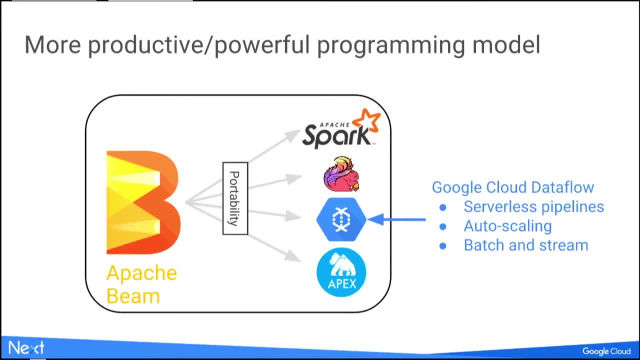 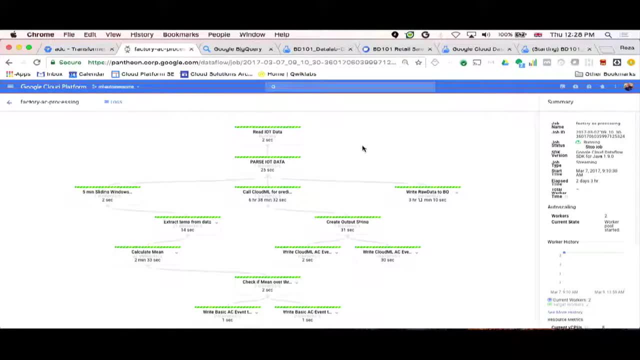 Now, very quickly, I'm going to show a demo of a Dataflow running, So if we can move over to the laptop, please. Thank you very much. So right now we're connecting to the monitoring UI of Dataflow And the example that's working is this. 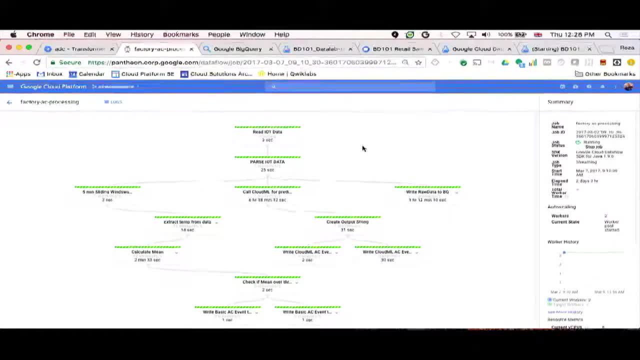 I'm working here for anyone who was at the session yesterday. This is an IoT example. There is messages coming from a factory. They have got temperature et cetera encoded in them. What we're doing is we're absorbing that through PubSub. 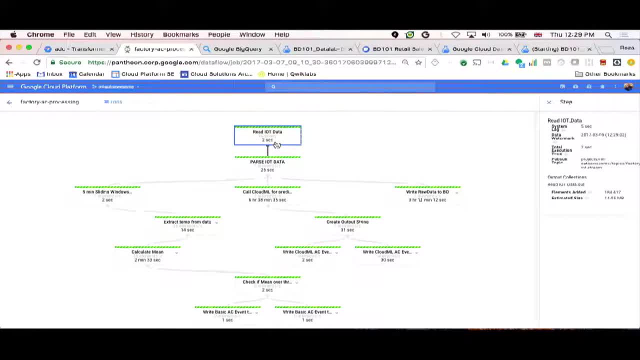 And Dataflow is pulling from PubSub. It's reading the IoT device data, We are parsing the message, We're pulling out little bits of information from the JSON package. that's there, And then I'm actually doing three different types of processing with that data. 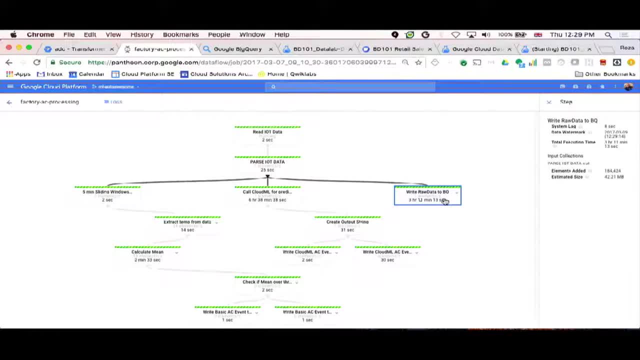 So the first one- and I'll consider this Like best practice always- is: before any processing, I want all the raw data to be dumped to a repository, And at this point we're putting it into BigQuery, because then we can run SQL analysis against it. 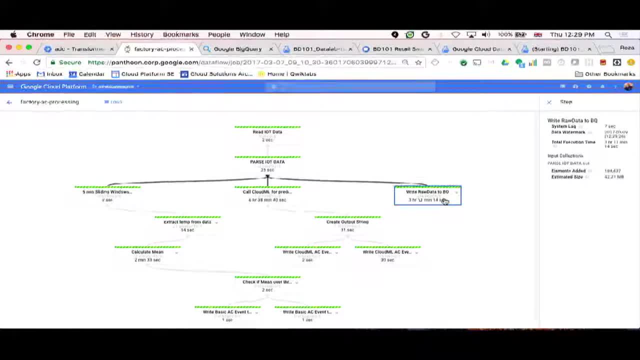 We'll come back to BigQuery in a moment- And on the other side we are doing some basic processing against the data. So here I'm creating a simple sliding window, That's two lines of code, Then I'm doing a mean calculation. 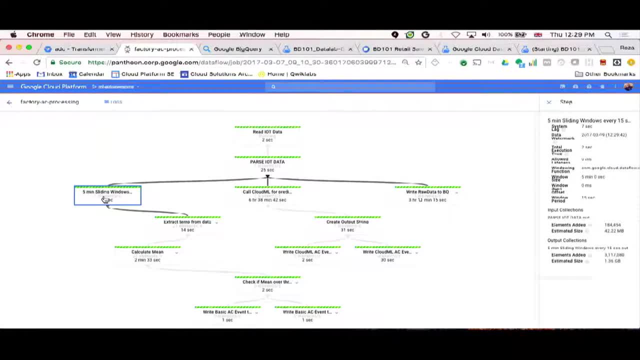 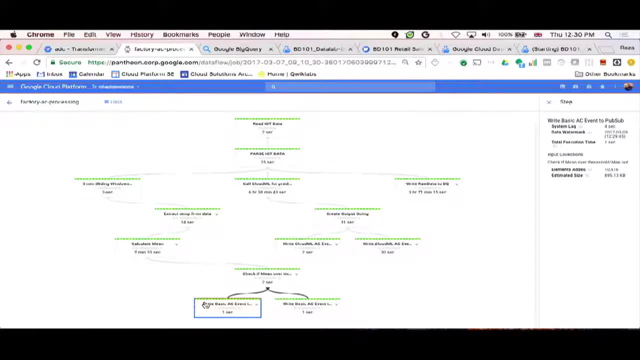 So, within the last five minutes, what was the temperature Then? I'm doing a very simplistic check. If the temperature was over 8,000, that's good for x. send the message back into PubSub. So here PubSub is not only being. 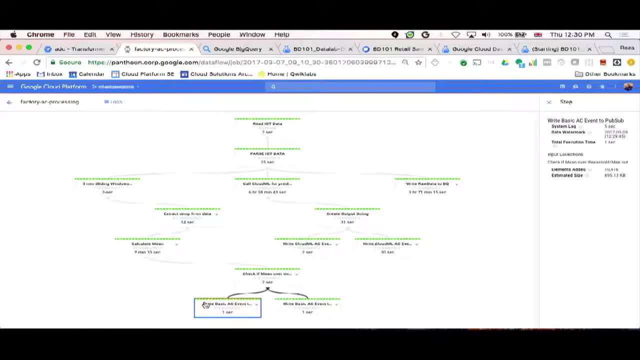 used as the ingestion mechanism into Dataflow. it's being used as the glue to connect systems together. So I'm sending a message saying AC on or off, and then the factory can pick that up. More interestingly, down this middle path, 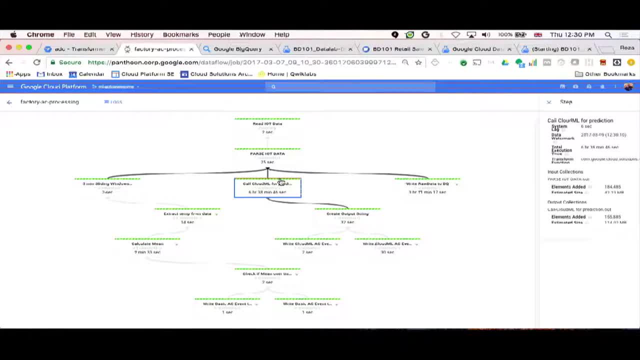 so that was a simple: is the temperature over 30 degrees? But down this middle path we actually called the Cloud Machine Learning Service. Here we have built a model based on data that would have been previously recorded in BigQuery, or that raw data that we should have recorded. 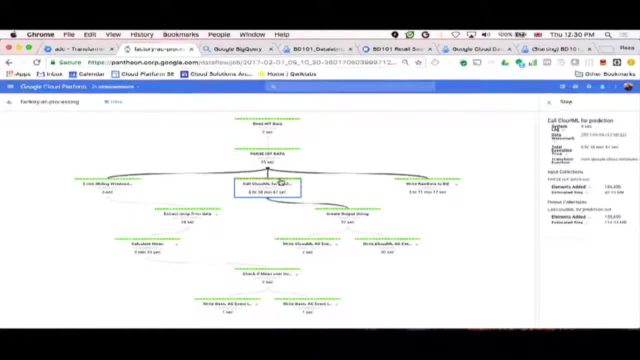 It is able to then tell us what the optimum time to turn the fan is on. So here, instead of making that simple check, I make a REST call to the inference service. on the model, It will tell me whether the fan should come on based. 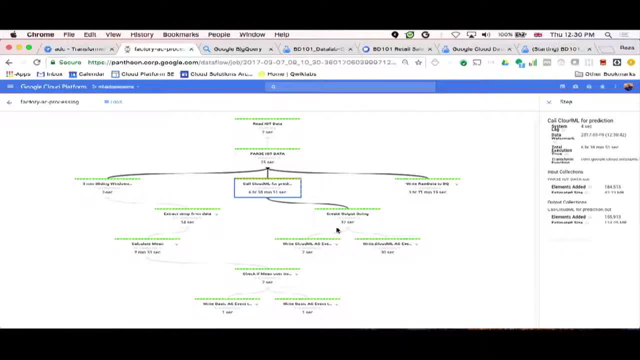 on the heuristics that we based on the cost optimization that we had in mind, which is efficiency, And it will. then again we put it back into PubSub to push back into our factories. We're talking heavily about retail use case. 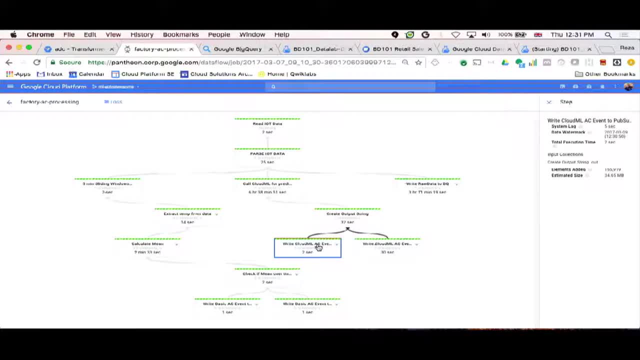 here with the sales data that William went through on Dataprep. A simple example for retail would be: take those IAT temperature readings and imagine they're actually coming from stores And what we're trying to do is what temperature should the store be set at to make sure people are spending? 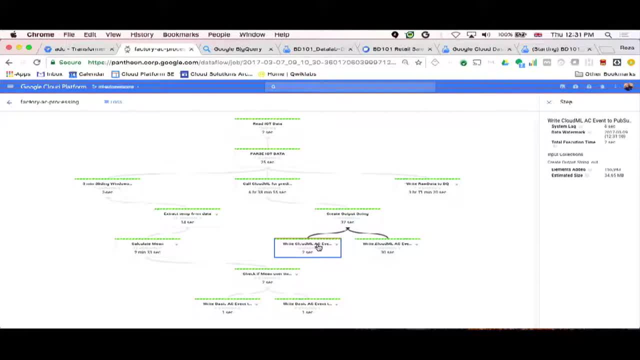 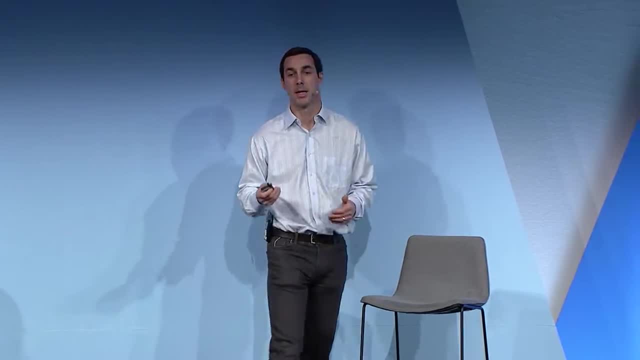 lots of good money in your stores. OK, Back to William WILLIAM SHATNER- Back to this slide, please. And so we talked about the difficulty of writing pipelines and how you can now, in many cases, not even have to write any code, or if you. 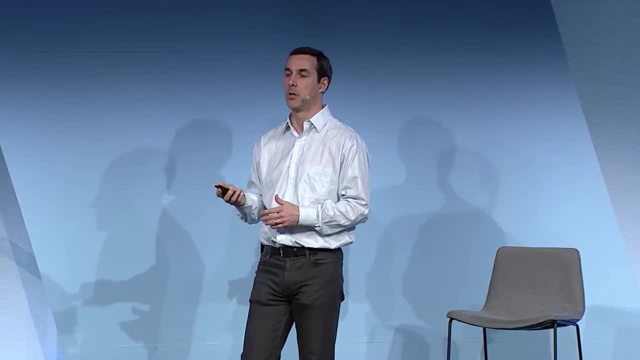 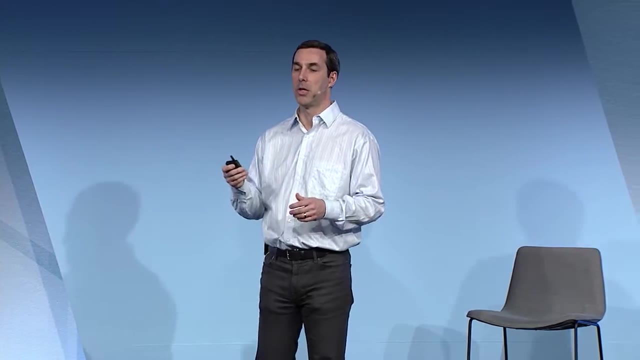 do have to write some code, have a very powerful and convenient programming model like Beam, running on Dataflow, which Reza showed. That really is only the tip of the iceberg, though, in terms of the complexity usually faced in terms of running big data in an organization. Quite often the hard part that comes after that is: how do you operationalize that? OK, you've written your first pipeline. How do you make sure? How do you make sure it runs at scale with just the right amount of infrastructure? 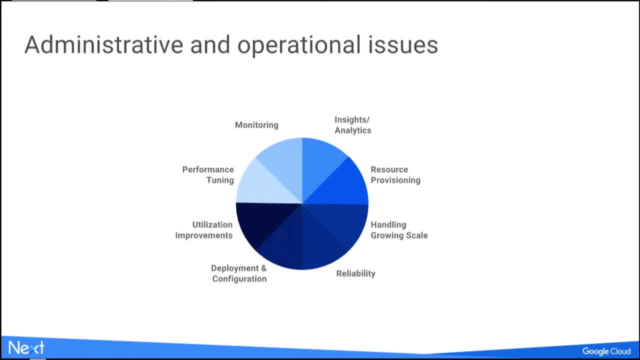 And that's often pretty complicated. And there are two main aspects there. One is the human aspect. It is a lot of work for people to have to deal with provisioning and patching and reliability and security and performance and optimization. 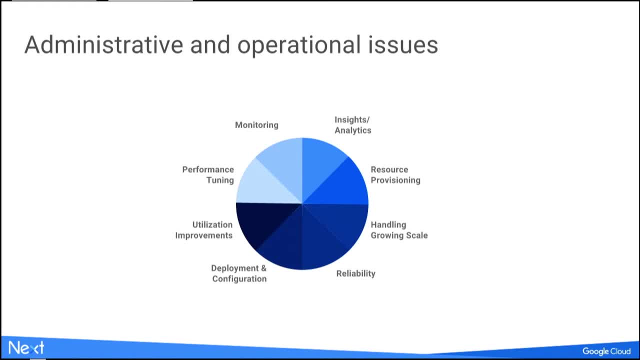 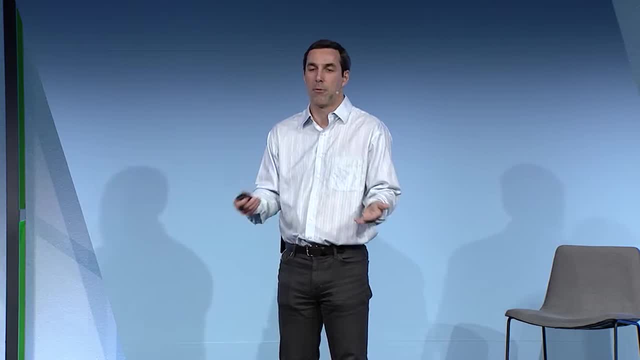 and all those operational aspects which you have to deal with, because, by definition, big data runs on a significant amount of computing power. You have to manage it efficiently, Otherwise you're spending way too much and it's just not doable. 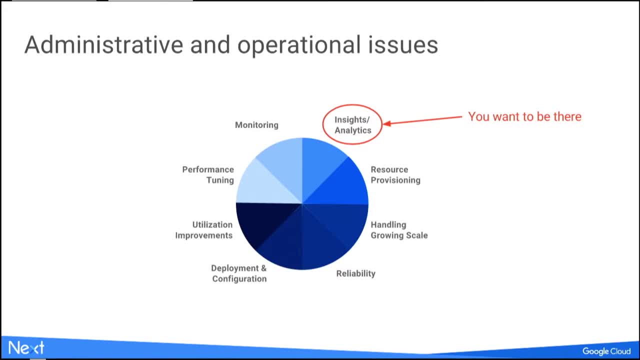 And so, in reality, this is where you want to spend your time is bringing your business expertise to the data, and not doing all the operation and trying to guess how much capacity you're going to need. And so there's a workload aspect and skill set. 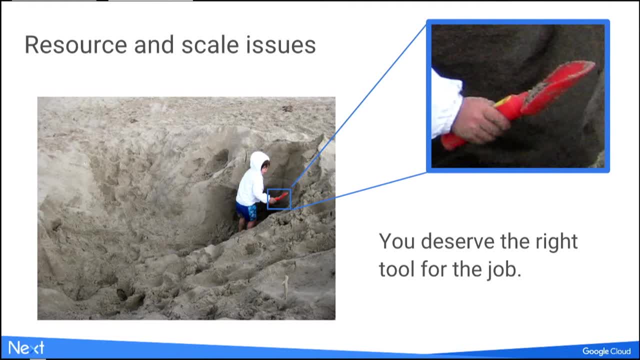 of constraints here. In addition to that, there is just resources. How often have you found yourself feeling like you have a tiny shovel And a really big job And you're not getting the resources you need, But that's because it's really hard. 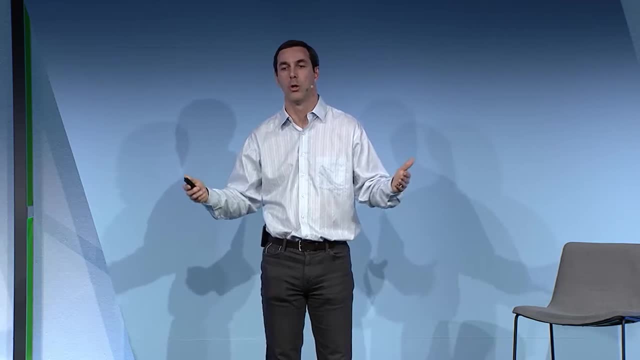 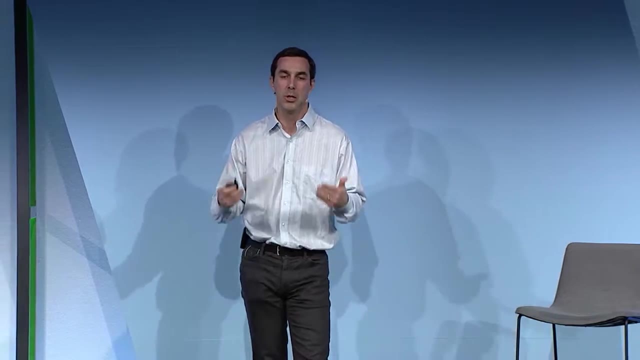 to get large amount of resources, at least until you know for sure what you're trying to get done. And the important thing is that you really want to encourage people to try things, to iterate, to fail quickly, to move on to the next thing. 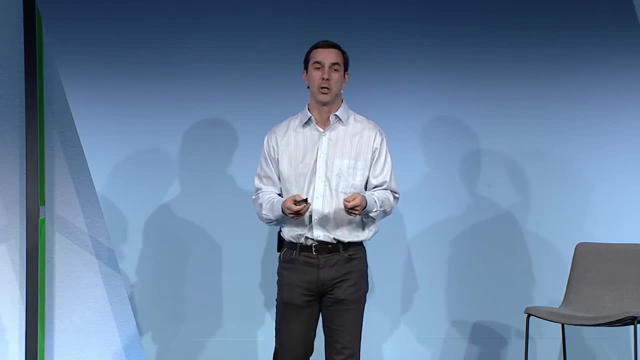 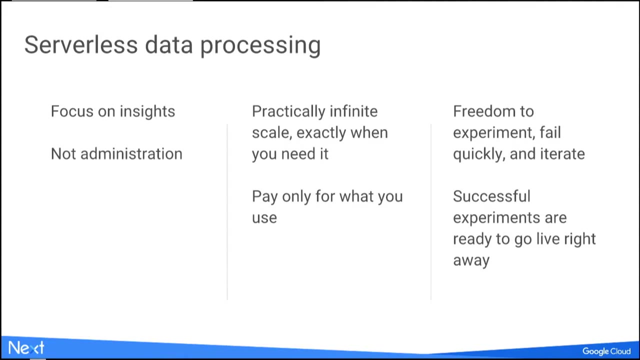 But if they cannot get infrastructure to support those experimentation, they're going to do toy projects, And the solution here is what the industry now calls serverless, Which is an approach to data processing that takes care of and automates all of the management and administration. 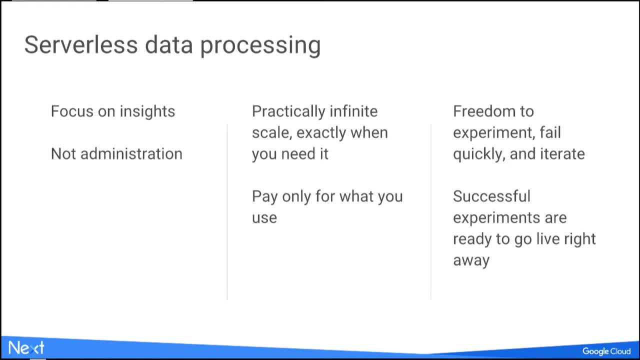 processes and allows you to focus on writing the job. So insight, business expertise, no administration. It also means that you get access to a lot of resources when you need them, but you only pay exactly for what you use, And so if you have an idea in the morning, 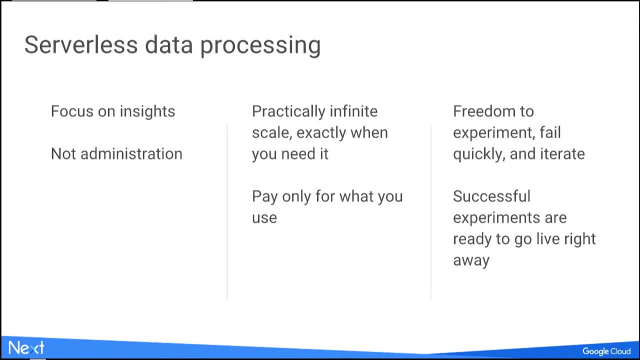 you can start and analyze large amounts of data to really validate your idea, And if it doesn't work, you've wasted an hour and $5 worth of processing. If, on the other hand, it does work, well, you don't have a toy project. 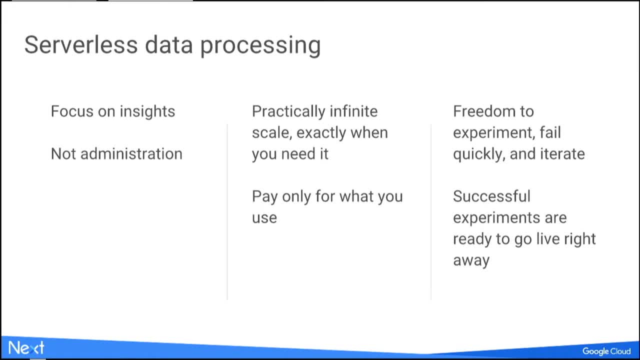 that you have to throw away and re-implement at large scale. You have something which is built on services that can natively scale to any size, And so any experiment that is successful is ready to operationalize and prioritize right away. And that's really the most important part. is not that? 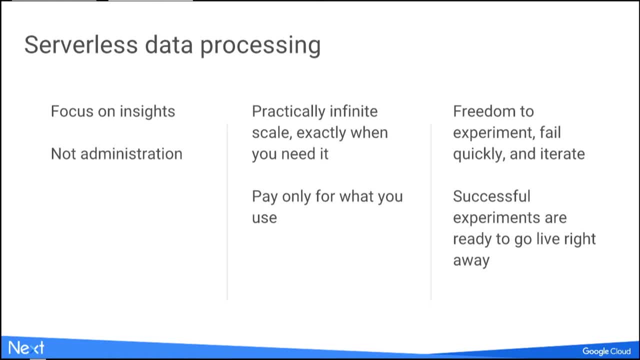 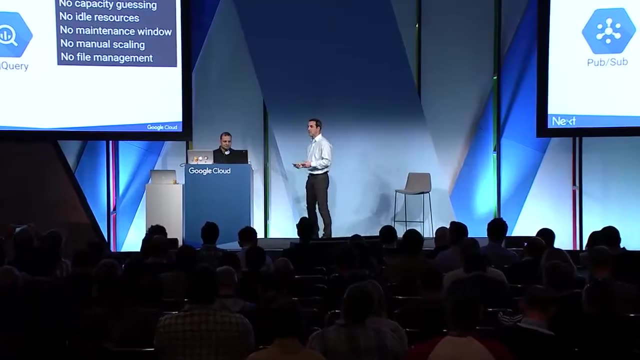 It's not the technology. It's really the way teams learn to work and test ideas and iterate very, very quickly, as opposed to any new idea being yet another IT project In practice. when I talk about serverless, well, there's many services on the platform. 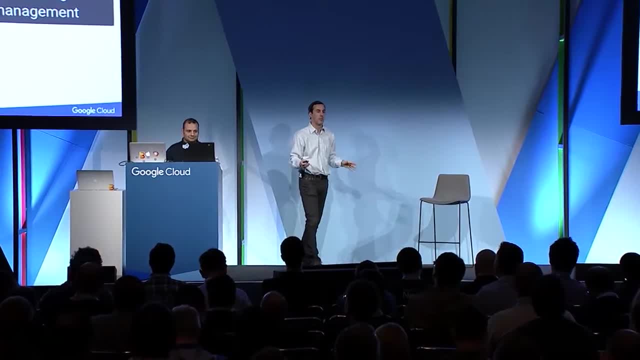 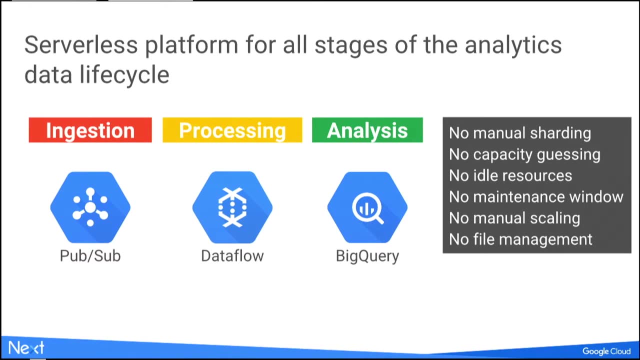 But the three that I would call out as the most obvious example have the NAS characteristics that they cover the three main stages of data lifecycle. And so Reza talked about PubSub. PubSub for event ingestion: Nothing to manage, Just create a topic and pump as many events as you want. 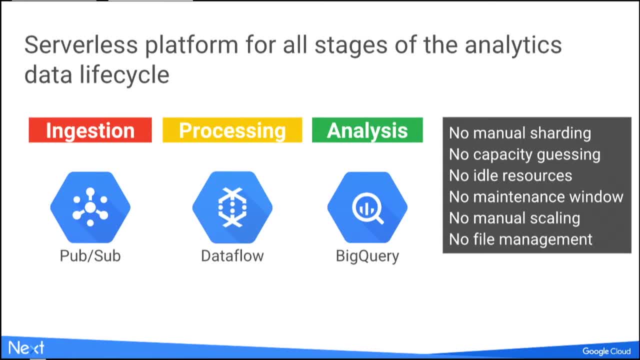 and only pay based on how much data you put through- Don't have to guess- and pre-provision ahead of time. Dataflow as well. Reza described the quality of the programming model, But the thing that's really unique about Dataflow. 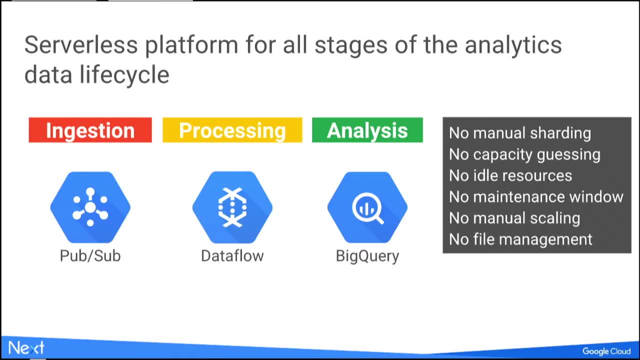 as a BIM runner is. it's a serverless system where you don't deploy a cluster. You submit a job and then the job automatically gets the resources it needs, autoscaled. So whether you use Dataprep to create that job or you write it yourself once you've created the pipeline, 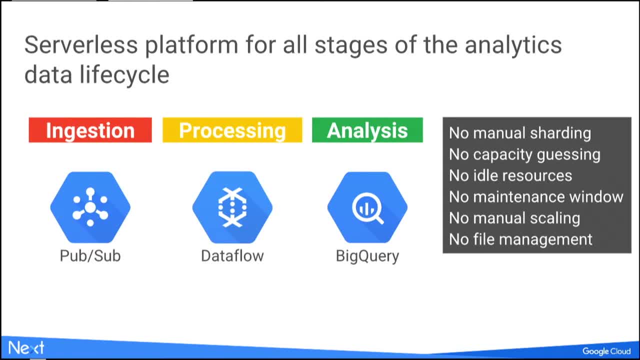 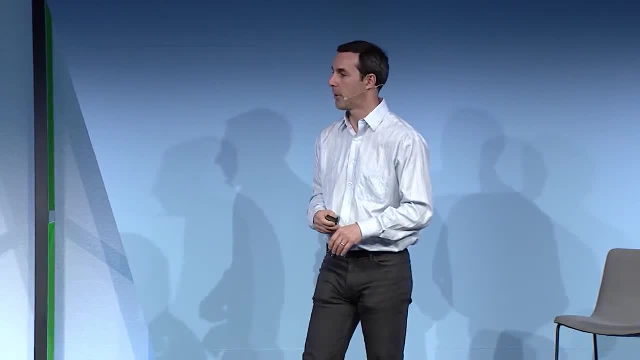 you're done, Everything else is automated. And then the third one which we're going to talk about now is BigQuery for SQL Analytics, Again serverless and at any scale. And so, Reza, please tell us about BigQuery. 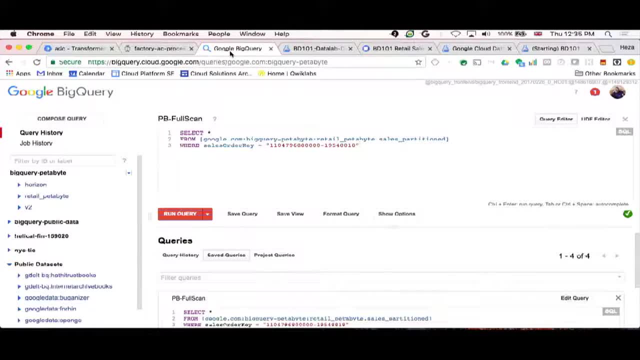 REZA SEYMOUR- Can we go back to the laptop, please? Thank you. So what we have here is the BigQuery user interface. I'm actually going to run a query which is a little bit unusual. We're going to run a query over one petabyte of data. 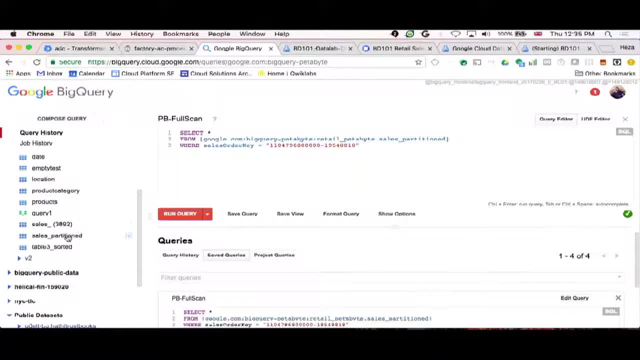 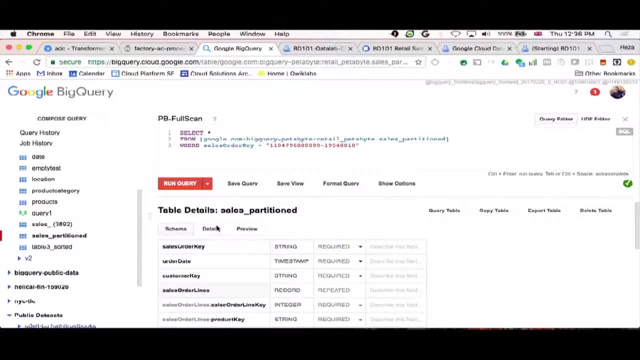 The table in question is a retail data set with a table sales partition. I can actually see the schema here. If I go to Details, we see that it is just over a petabyte of data in volume and around a trillion rows- well, just over a trillion rows. 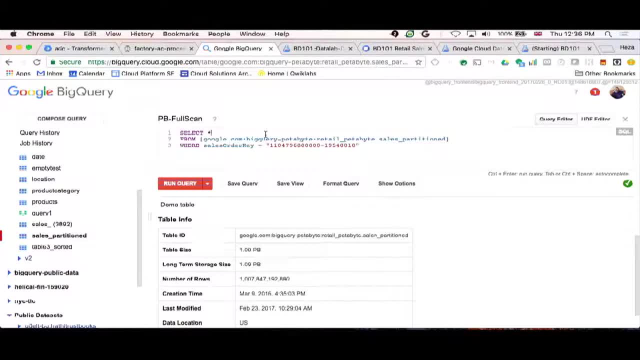 to compute. Now, BigQuery is a columnar iOS storage format, So we don't, and actually it's been moved to Capacitor since its first inception. but here I'm going to do a select star, which is a bit of an unusual thing to do here. 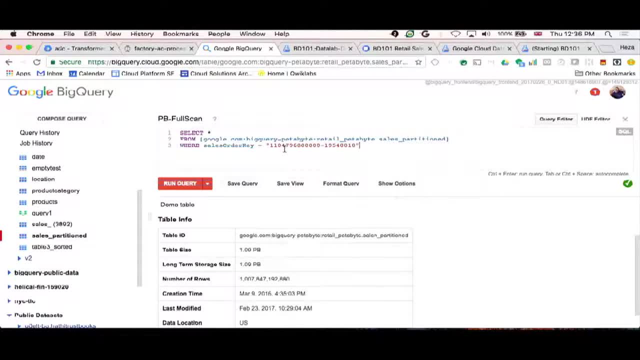 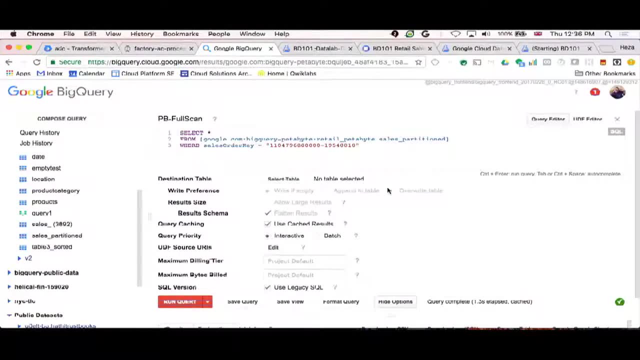 and look for a single predicate. This is just to force it to compute against the whole data set, So I'm going to kick that off and get it to run. That will take a few minutes to actually sorry, that's been cached. 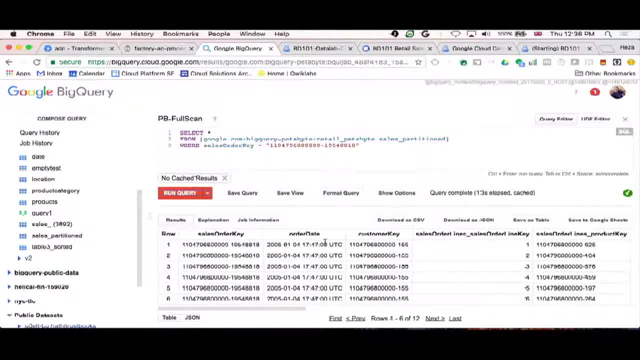 Let me remove the cache, So BigQuery will cache results if you've run it before. Obviously we don't want to do that, So let's get it running properly. So that's now going to run. It's going to take a few minutes. 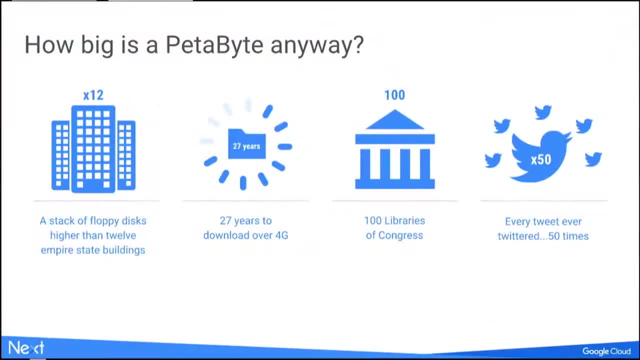 If we can go back to the slides please. So let's think about what actually is a petabyte. So I'm going to show my age a little bit here and talk about floppy disks. So if you wanted to store a petabyte onto floppy disks, 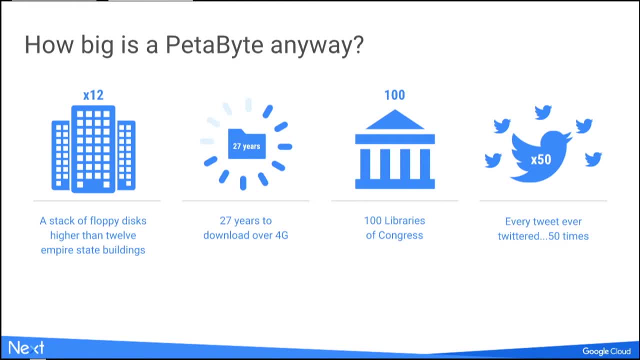 you'd have to stack up 12 Empire State buildings worth of them. It would take you 27 years to download over 4G, And it's every tweet ever made times 50. But that's a big number, obviously. petabyte. 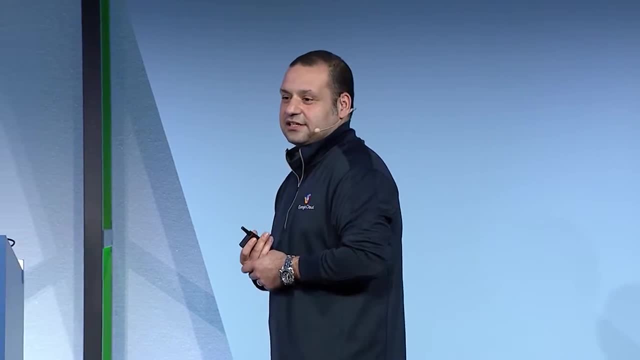 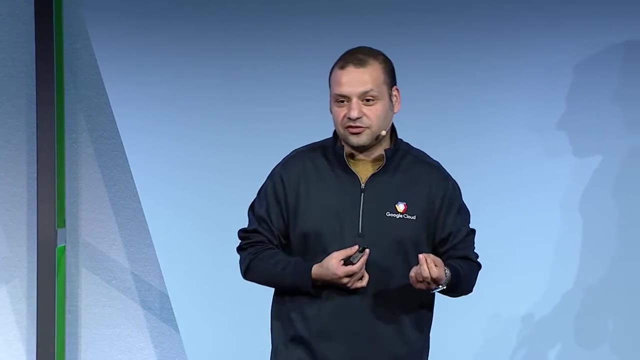 But it can also be a small number. So it's the data that's encoded in just two micrograms of DNA. It's one day's worth of YouTube video. It's 200 servers logging at a fair pace, admittedly- 50 entries a second for three years. 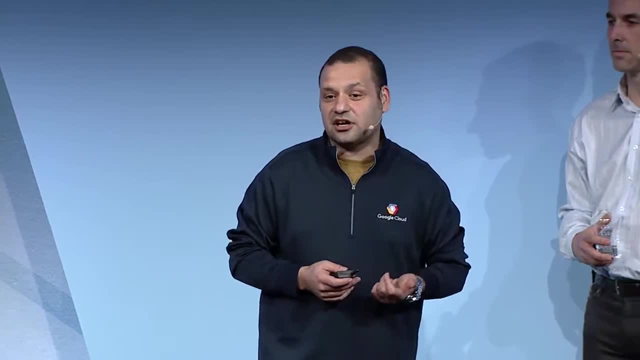 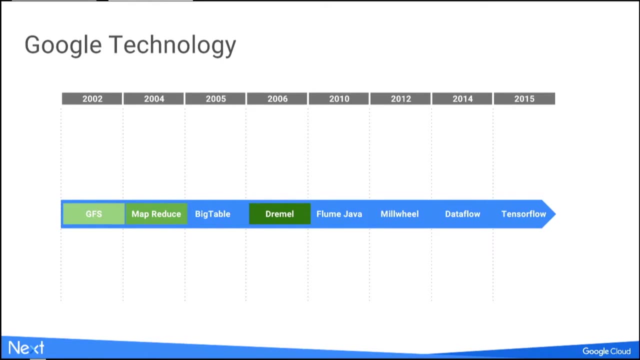 So there's going to be more and more data sets that actually have these kind of volumes of data as we move forward. And where did BigQuery come from? So BigQuery is based on a technology called Dremel, And in 2002, Google had more and more data to store. 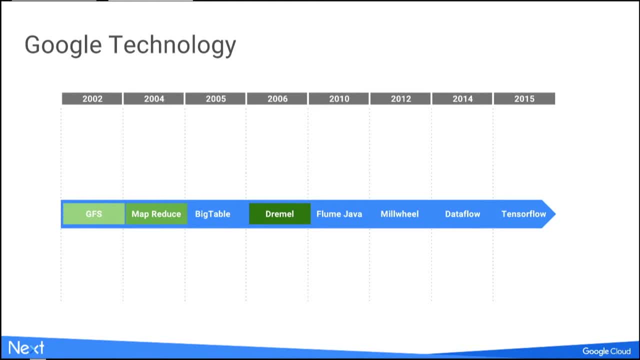 And the Google file system was bought. It allowed you to store all of this data in commodity servers- Fantastic. We solved the problem of how to store lots of data By 2004,. we had lots of data And we had to figure out the problem of how. 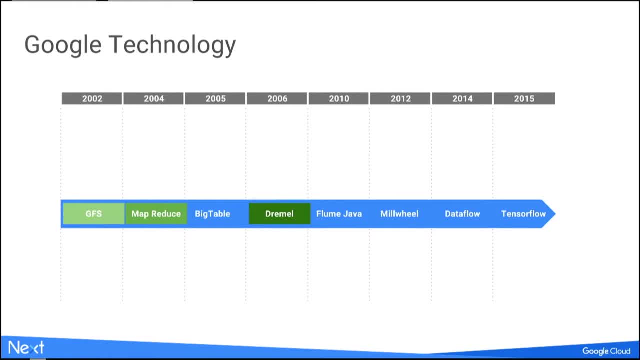 do you process all of that data? So, Jeff Dean and co. MapReduce was used- And it was very heavily used- to actually be able to process all of the data that we had. Now, when you're doing analytics, you don't just write the perfect query at the end. 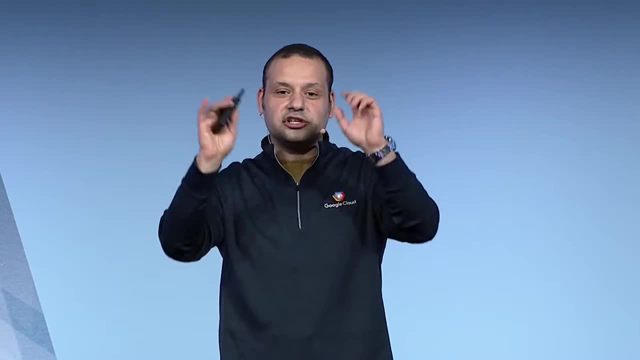 You know you wake up in the morning and you've got it all ready for you. You will look at your data. You want to analyze it. So if you're doing a MapReduce, you'd have to do some analysis with the first MapReduce. 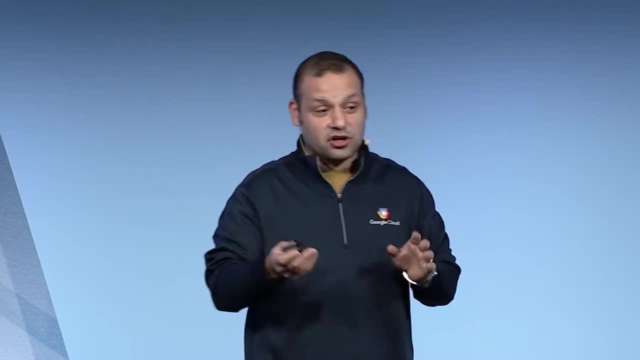 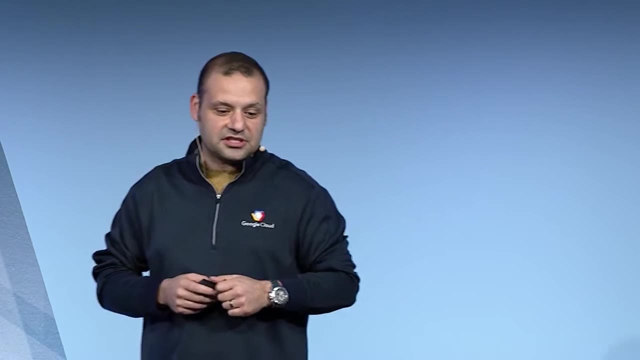 Then you would take the result set. look at that, do another MapReduce. And so our engineers got kind of bored with going off for coffee every time. they ran that first MapReduce and building all the plumbing in between this stuff and they wrote Dremel. 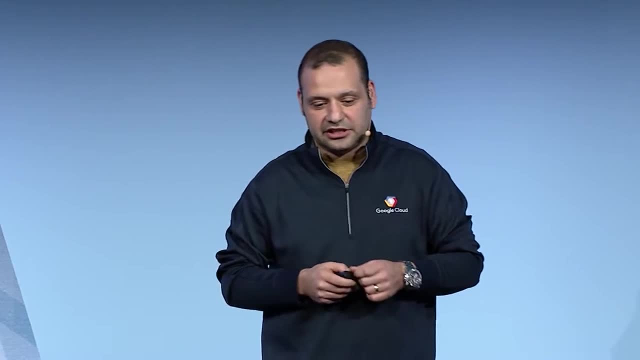 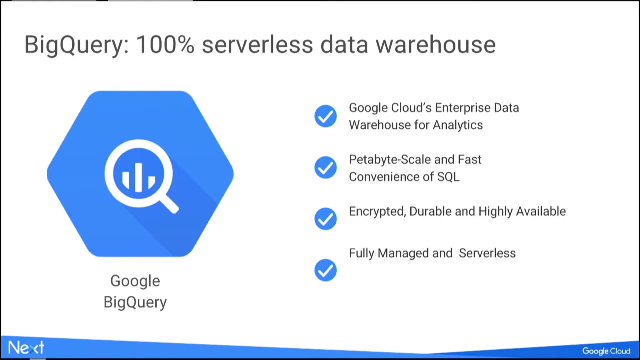 And Dremel allows you to run queries against petabytes of data, as we're doing in the demo now, And it's the same technology that has been externalized as BigQuery. So it's the same code base, It's the same SREs. 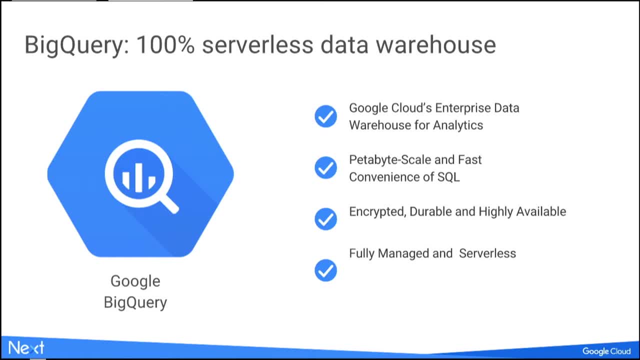 It's the same engineers And within Google. today, Dremel is the core of our ad hoc analytics and web data warehousing needs. Most Googlers will touch it- Myself and William will touch it more directly. things with Dremel. 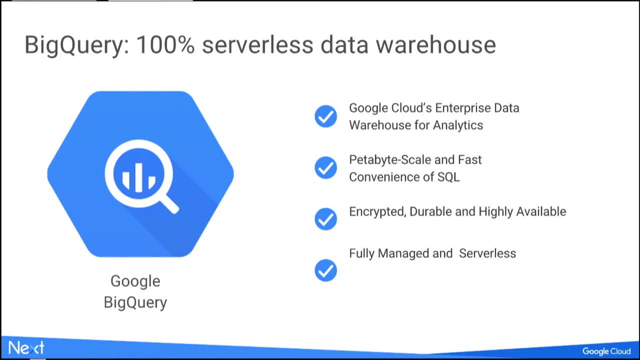 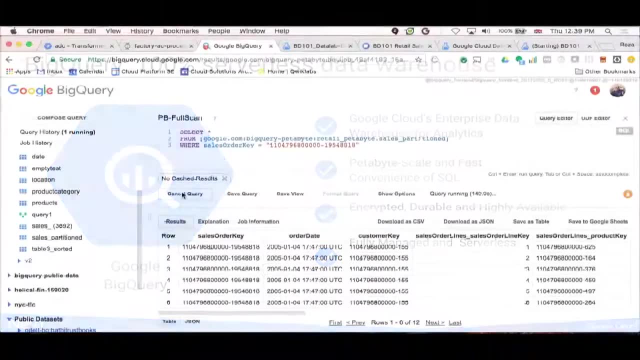 But, however, other people will be using it through dashboards, So now, OK, this query is still running. For now, we're going to switch back to William WILLIAM BONVILLIANI- Can you talk about the second? 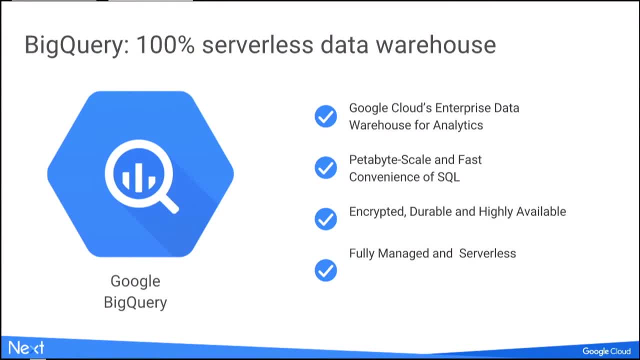 Go back to the slides, please. You talk too fast. CHRISTIAAN BRINKHOFF- I do sorry, WILLIAM BONVILLIANI- And so, speaking of the data and the way it's being stored and queried, 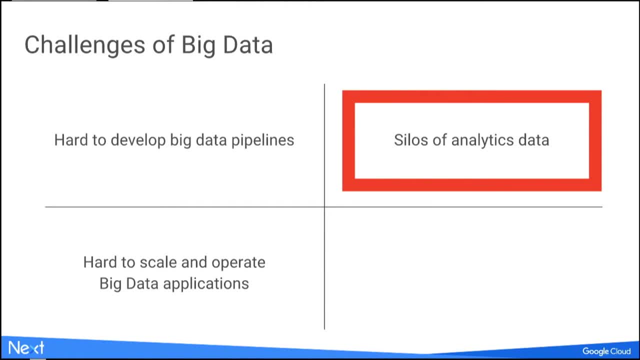 in Dremel, at Google. at Google, we have lots of different storage systems and lots of different processing systems. You want to go back to the slide for a second? CHRISTIAAN BRINKHOFF- Sorry, yeah. WILLIAM BONVILLIANI- Go back to the demo for a second. 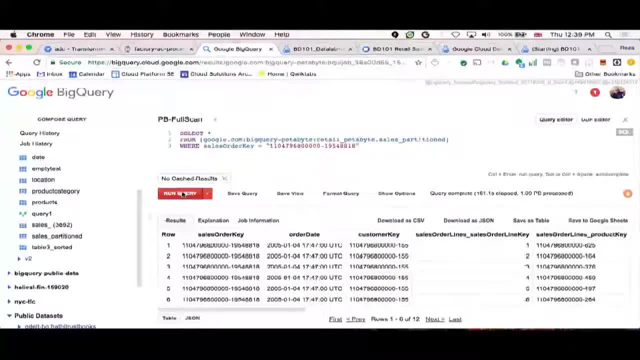 CHRISTIAAN BRINKHOFF- So I just needed to slow down for 20 seconds and it would have been fine. So if we go back, that query completed. It processed a petabyte of data. It took 161 seconds to complete. 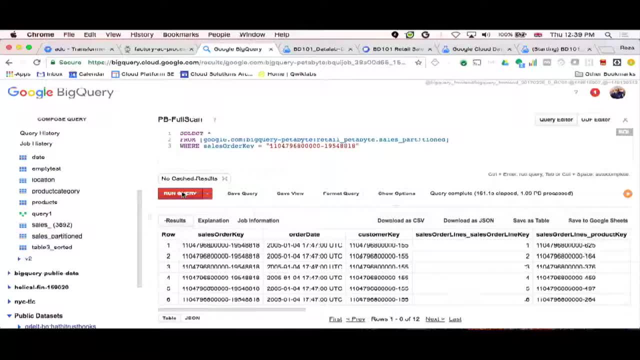 WILLIAM BONVILLIANI- That's 2 minutes and 40 seconds. CHRISTIAAN BRINKHOFF- Yeah, WILLIAM BONVILLIANI- All right, Thank you, CHRISTIAAN BRINKHOFF- Back to the slides, please. 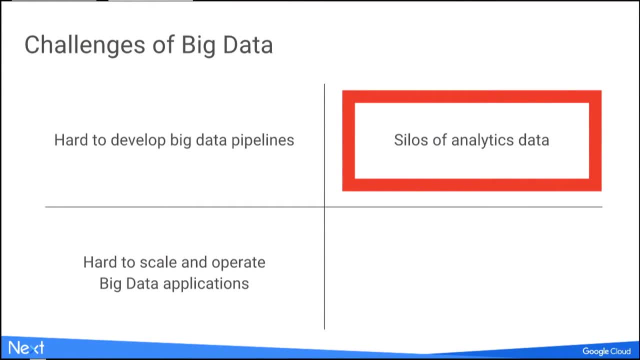 So back to the slides. So one of the other issues that's been preventing or making it harder to access and analyze data at scale is the siloed nature of the data, the fact that quite often data is within a tool And if you want to use another tool to process it, well, 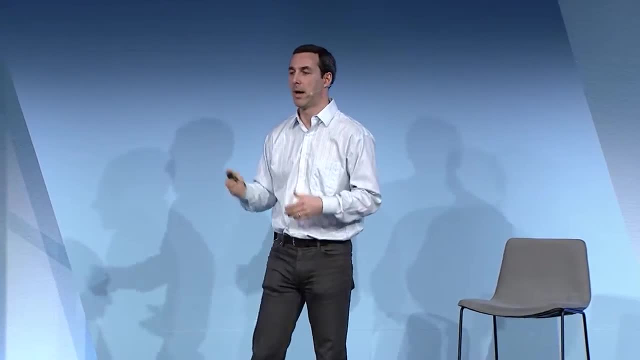 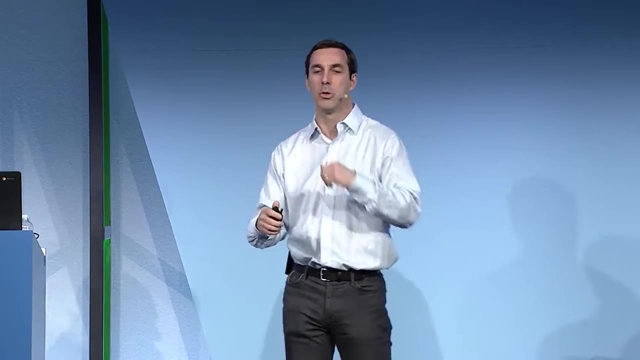 then you have to extract it, move it, copy it, have different versions, And at Google we have lots of ways to store data and lots of ways to process data and lots of data between the two, And if we had to do that, that would just. 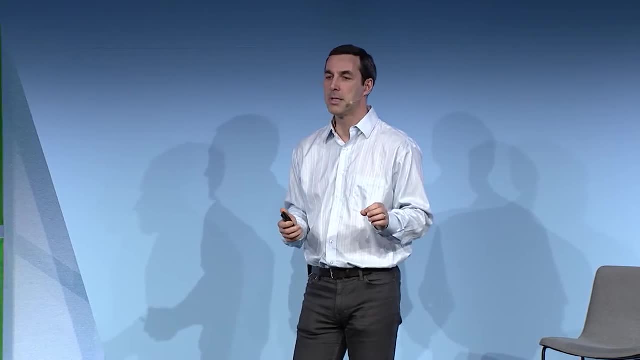 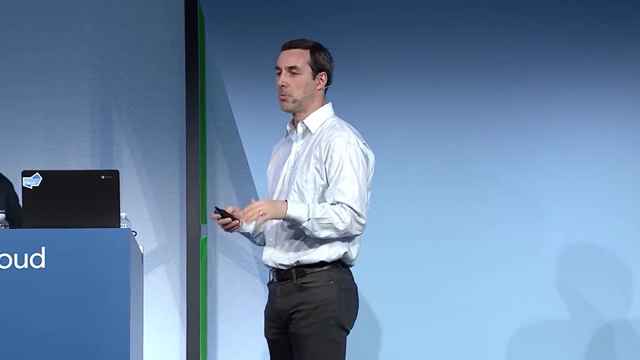 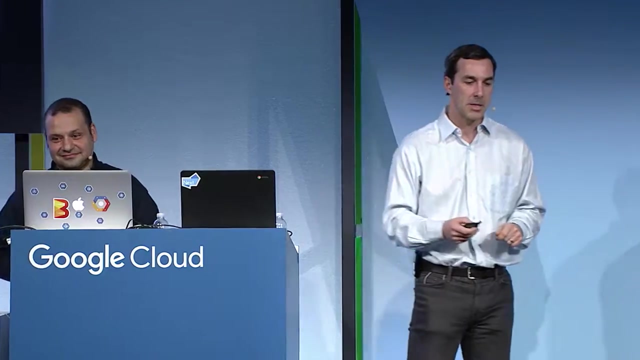 explode the data center, And so one fundamental principle is that any tool can access data in any storage, And that's really really important in terms of allowing a much broader analysis across sources of data set And so in cloud, the way that materializes itself. 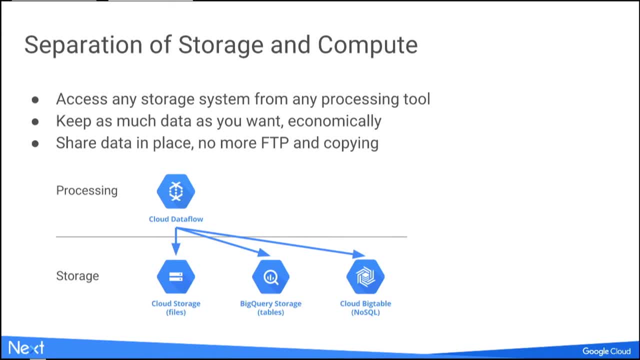 is, with something like Dataflow, which Reza described, being able to access data in Google Cloud Storage, in BigQuery, in Bigtable- That's our NoSQL service- in Datastore, all the databases that we have in PubSub for EventStream. 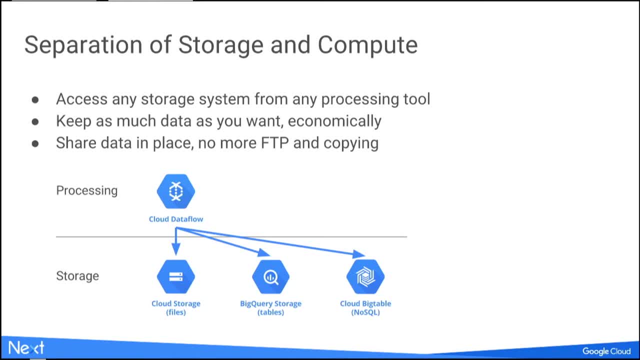 Wherever data is, Dataflow can get it and process it. Now it's maybe less intuitive, but the same thing is true for BigQuery as well, And so if you're going to try to go through a petabyte of data in, was it two minutes and 40 seconds? 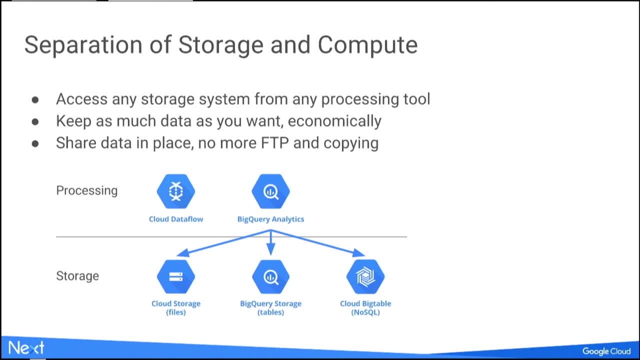 you have to put the data in BigQuery storage because it's highly optimized storage system for analytics. But in many cases you don't have petabytes of data And it might be more convenient to leave the data elsewhere as a file in Google Cloud Storage in Bigtable. 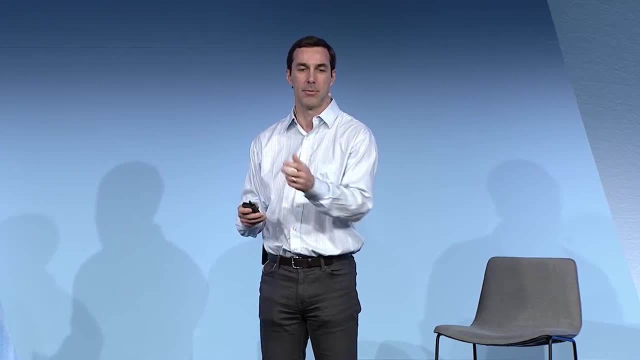 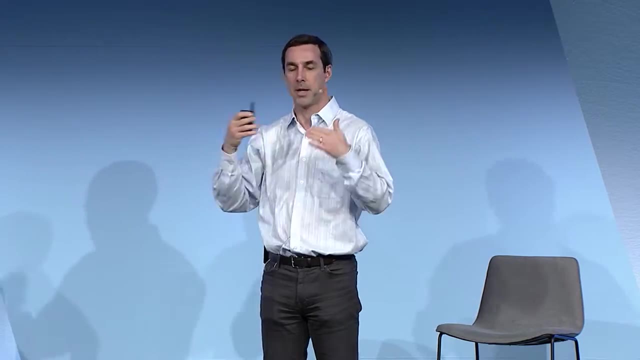 or maybe just even in Google Drive. So in my laptop I can have a CSV file which I drag in my Google Drive folder. It gets synchronized to Google Drive And now I can write a BigQuery query that is going to join from that CSV file in Google Drive. 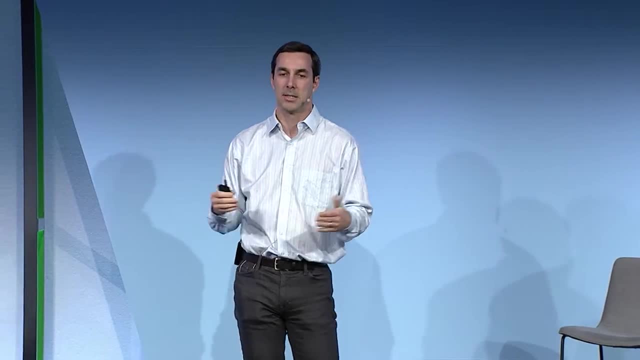 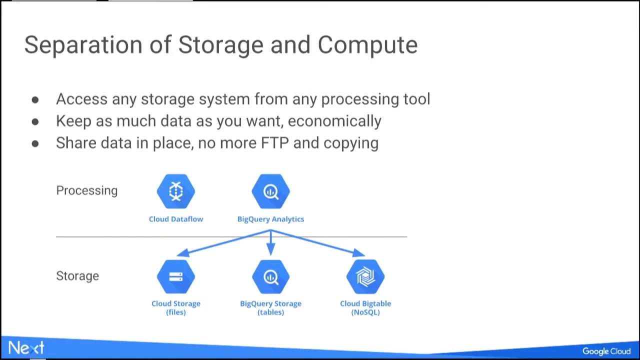 with, maybe, a log table in BigQuery, And so BigQuery has that functionality. It can bring SQL analytics to all the structured data on the cloud. And then, finally, another product we haven't talked about yet: it's Dataproc for managed Spark and Hadoop. 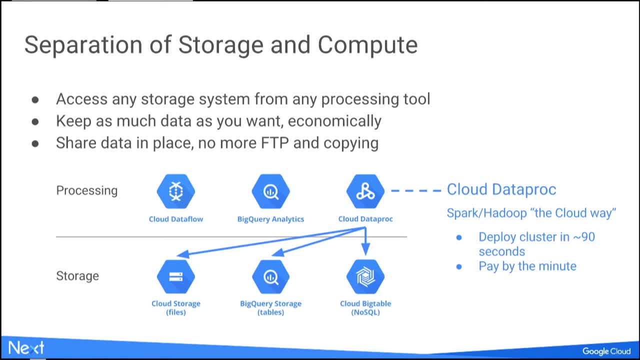 What it allows you to do is to bring the power and richness of the Hadoop ecosystem and Spark ecosystem to Google Cloud, Because the key thing is use the right tool for the job, And if the right tool is a Spark library that somebody wrote, 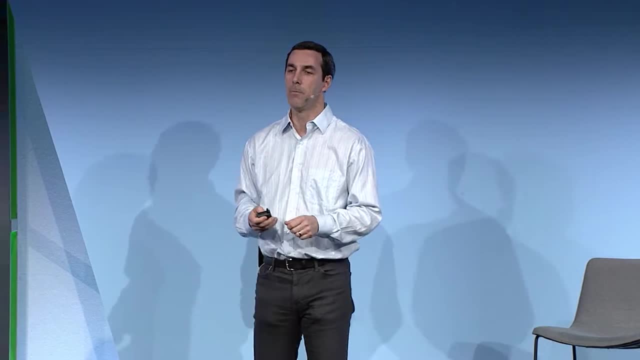 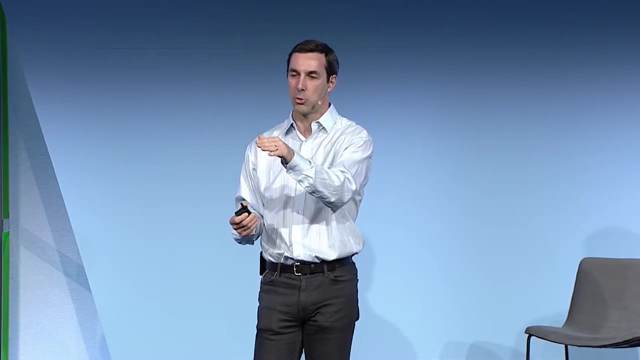 then you should be able to use that And Dataproc will give you a fully configured cluster in about 90 seconds And that cluster will have direct access to data again in the storage system, such that the first thing you do is not. 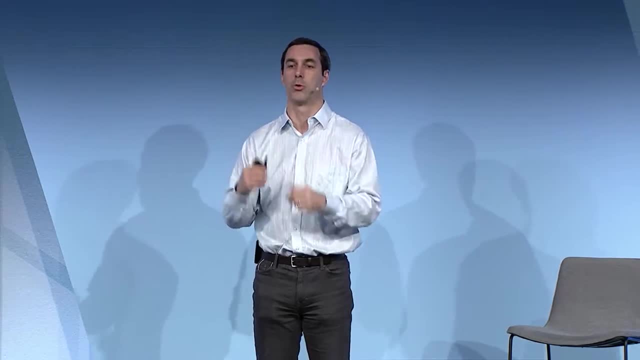 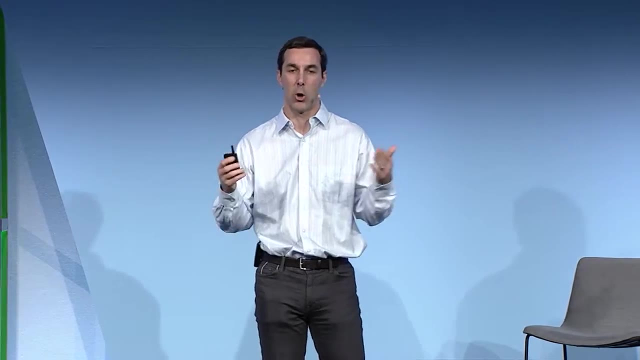 load the data. in Hadoop, The first thing you do is run the job, And so you can start a job run, shut down your cluster when you're done and you pay by the minute, And so it's standard Hadoop and Spark. 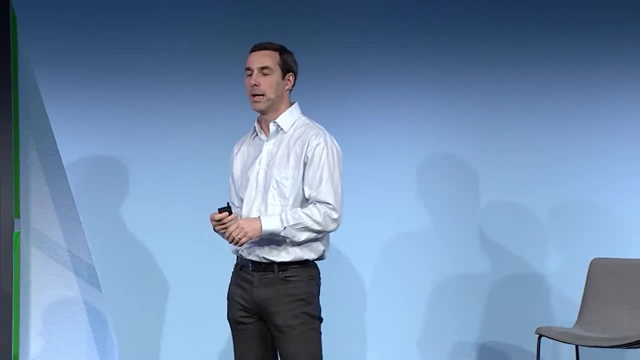 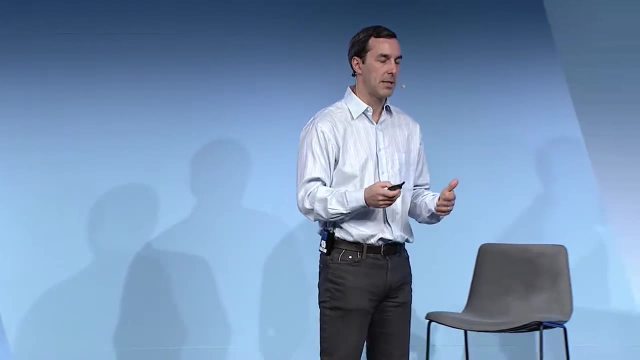 but it enables them to run in a very dynamic, efficient, cloud-native way And again accessing your data wherever it is. And then, finally, the last set of issues that people typically run into is just the tooling to do something useful with the data. 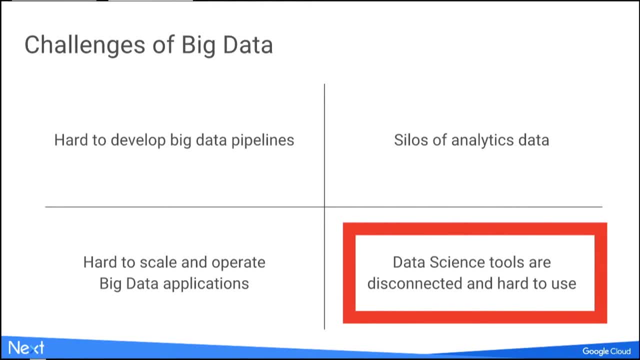 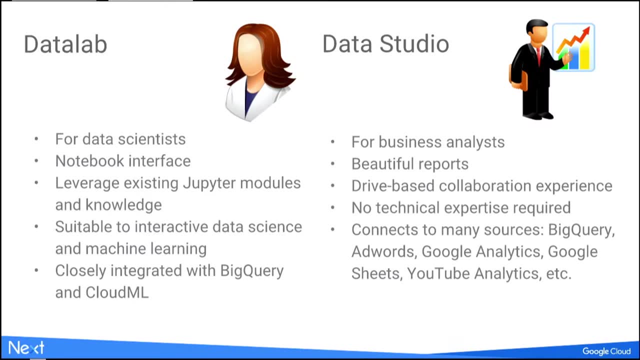 Because, at the end, it's nice to be able to collect it and process it, but to what end? And going back to the use cases, quite often that end is to inform a human, And so there are tools that help you do that. 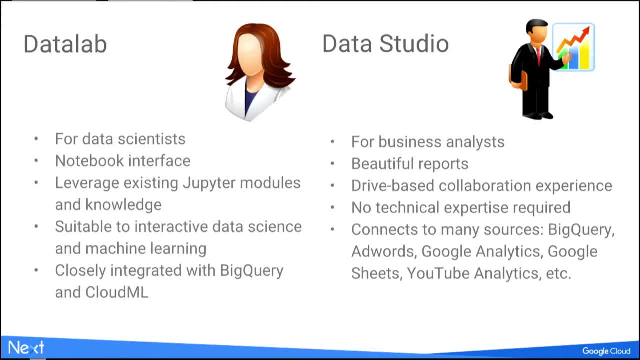 On the platform. specifically, there are two main tools which are directly accessible. One is Datalab. Datalab is targeted at data scientists, And so, for data scientists, Jupyter notebooks are a very popular way to analyze data And what Datalab is, is Jupyter closely integrated? 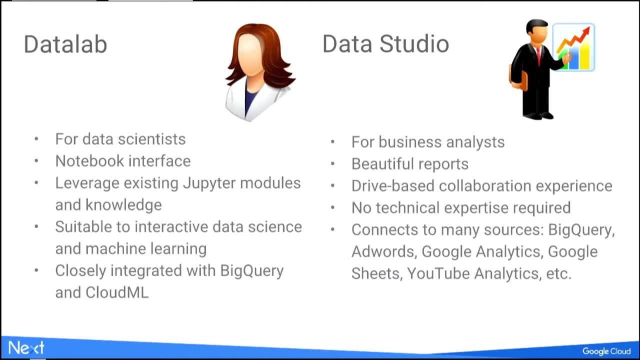 with Google Cloud Platform to allow data scientists to benefit from all the Jupyter modules and experience, but do that in a way that enables collaboration and usage on the platform, And Reza is going to show that in action. REZA SAYAHIRI- Yeah, and so the interesting thing. 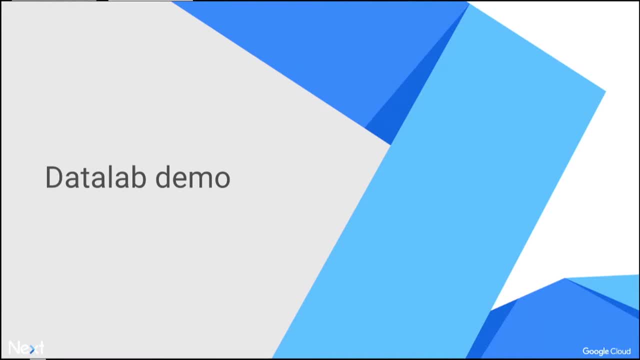 about notebooks is it's the data scientist's kind of scratch pad. As they're going through and analyzing the data, they can just record their results. They can go back to them, They can use that even as something that you pass to the data engineers- that's me. 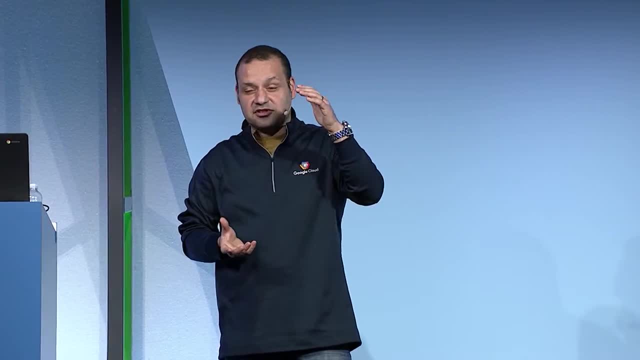 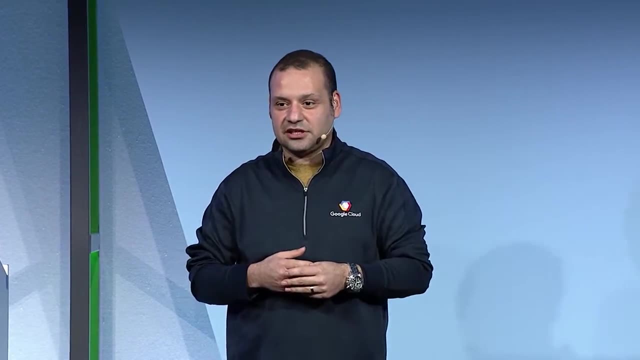 to actually go and put into production. And the other thing, the great way that I've seen them used is at the end of their conclusions, after they come to what they think is the right way forward, they'll present the notebook back to their colleagues. 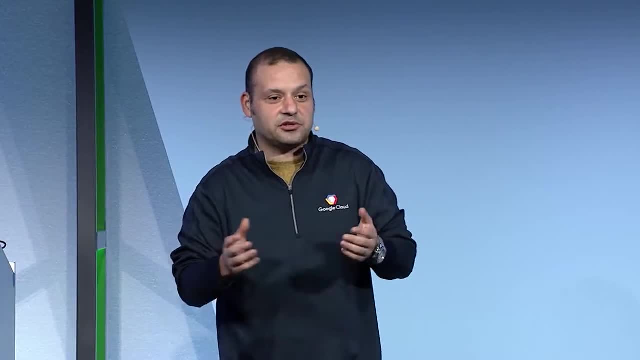 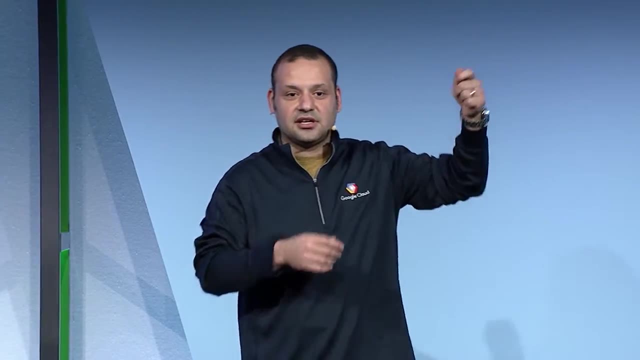 And that's great, because at the end, when they have that final result, you might have a question like: why did you use column A and not column B? And they'll go back and say: well, actually I looked at column A and I saw a skew in the data. 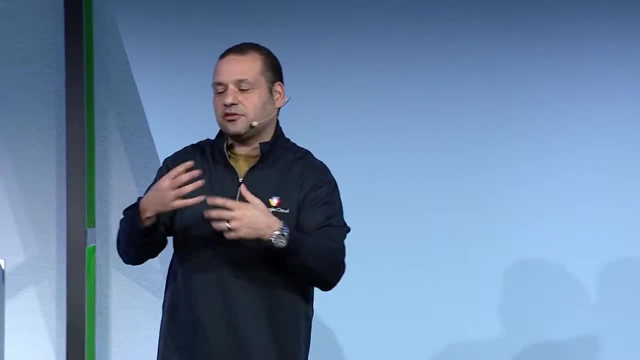 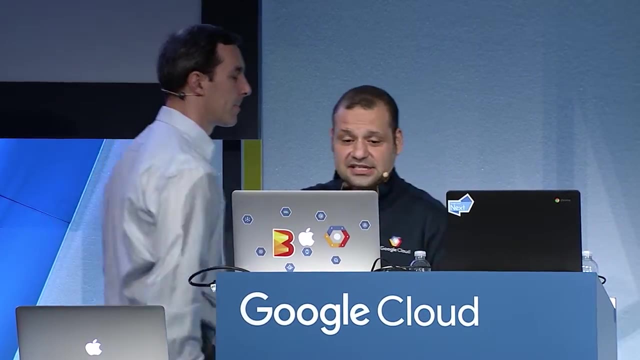 Therefore, I switched to column B, And it's a great way to actually maintain all of the knowledge that you gain as you explore your data set. So if we could switch to the laptop, please. What we have here is a data lab, that's. 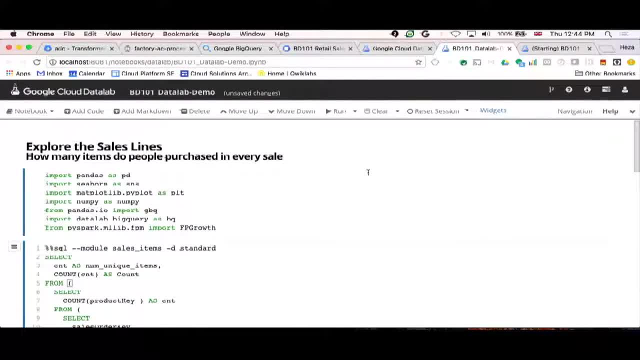 been set up to run in Dataproc, our managed Hadoop and Spark, And what I'm going to do is actually use the data lab in conjunction with BigQuery, with Spark, to actually do some simple analysis against that sales data. 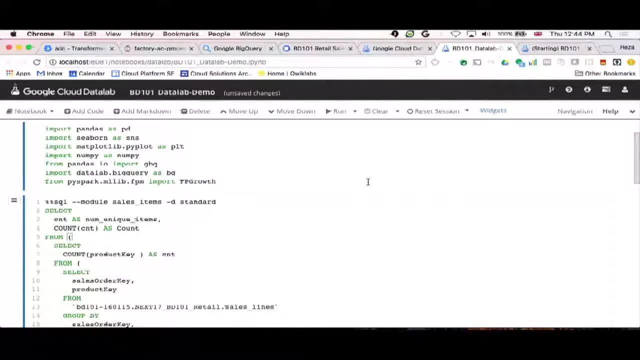 So what I want to do is, as you can see, it is a hands-on kind of technical tool. What I'm going to do is look at the sales information And the first question I'm going to say is: OK, so let's figure out how many items. 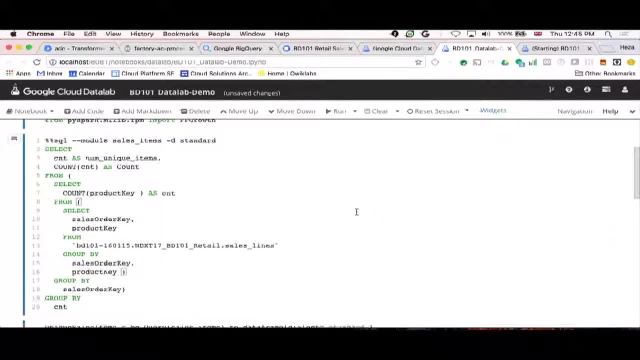 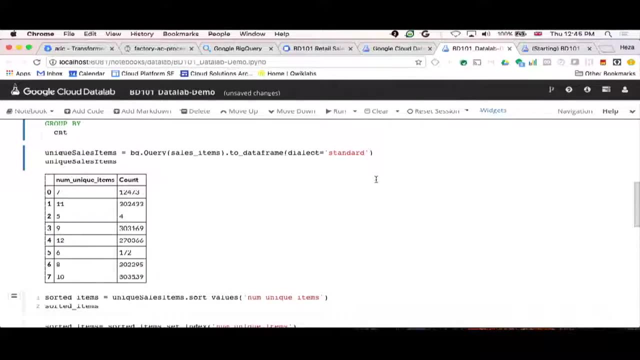 there are in an average basket. So I would write a bit of SQL, run that cell. I would then call the BigQuery connector. It's gone and actually used the power of BigQuery to do the hard computation. It's given me back a table with eight rows. 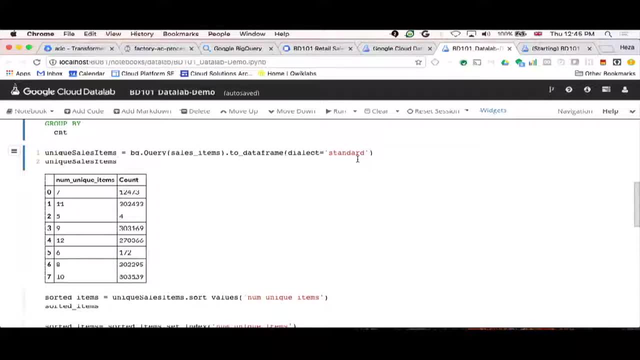 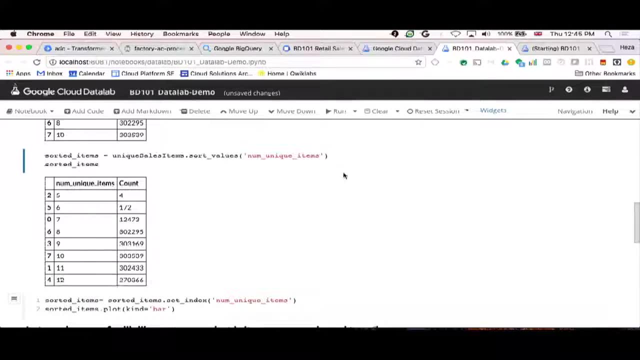 Now the eight rows weren't sorted so I could go and rewrite the query with an order by, But actually, as I'm in the notebook, I'll just use the sort from the data frame. Great, I can actually see now that in general there. 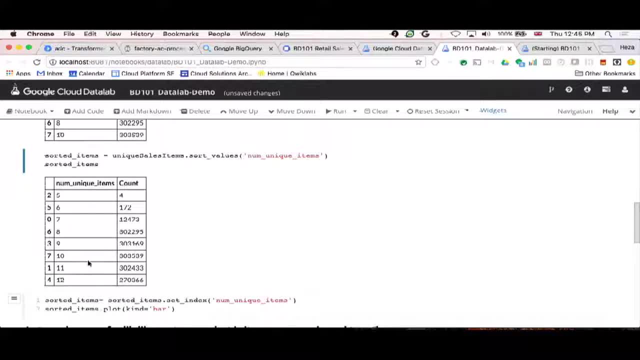 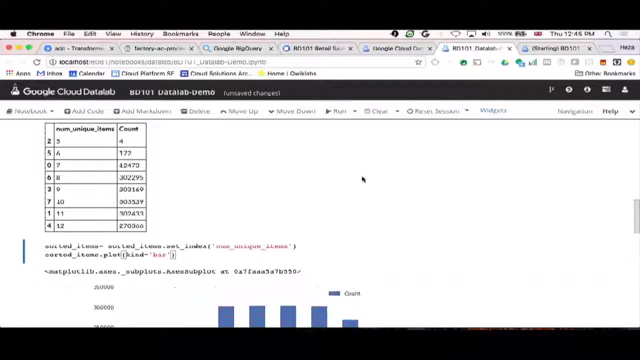 are number between 8 and 11,. it seems to be the average number of items that we're going to have in a basket. OK, interesting, Let's start doing a plot- a favorite tool. So great, we've got a visual representation of that data. 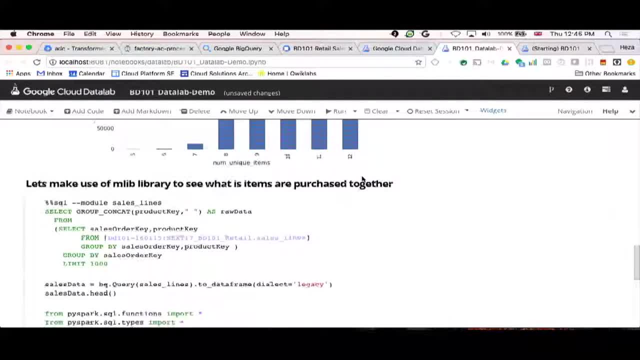 Let's move on to something a little bit more tricky. So what I want to do now is figure out what are the things that are actually bought with each other. So that would be incredibly difficult to do with something like SQL, because you need to get the power set of all the items together. 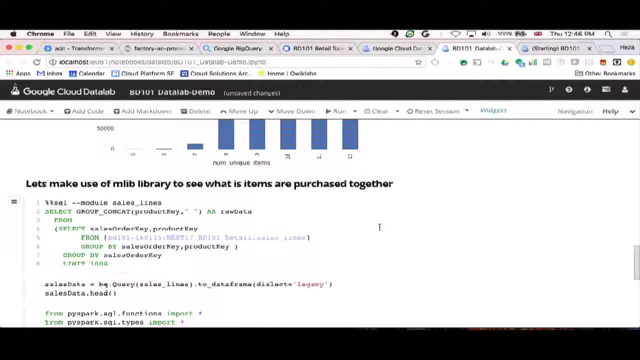 So what I'm going to do is make a combination usage of BigQuery plus some MLib library algorithms that exist in Spark. I'm going to get the data ready in BigQuery. So what I'm doing Here is generating a set of data for this demo. 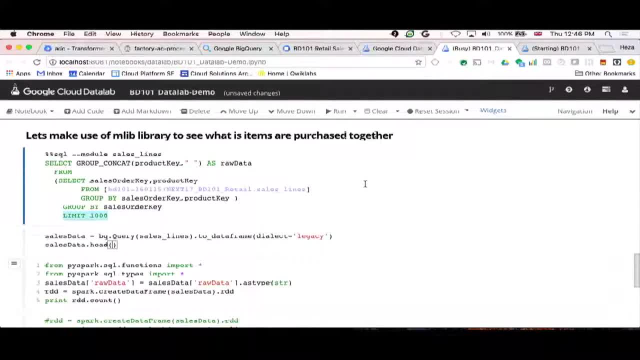 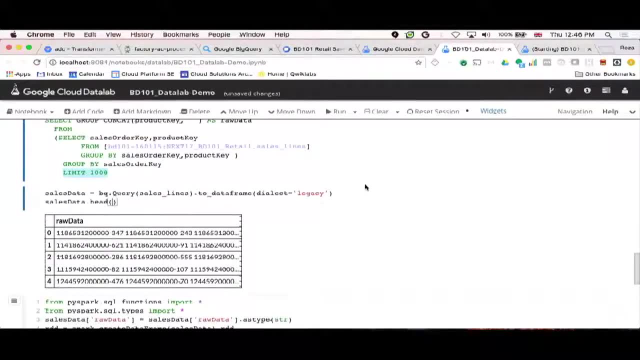 I'm just limiting it to 1,000 rows to return And if we look at that head, what that's done is it's gone through all of my sales data and just concatenated all of the product IDs- the same product IDs you were seeing when William was running. 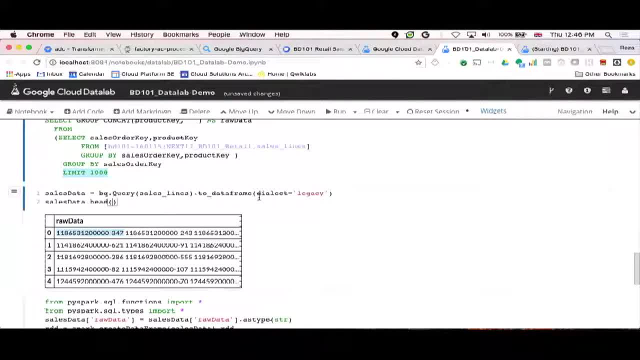 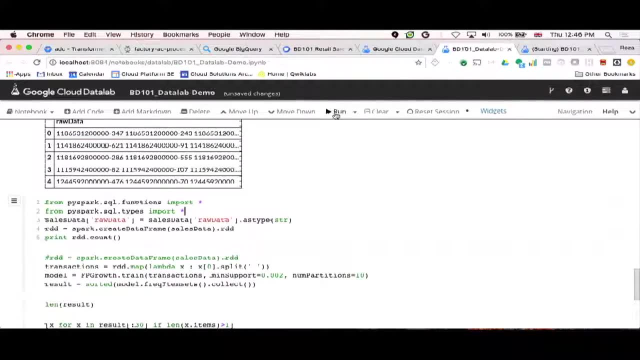 the Dataprep demo. So it's put them all onto a transaction line. This is now perfectly ready for my algorithm, So I'm not having to do any work in Spark to get the data ready. So now I'm going to run. 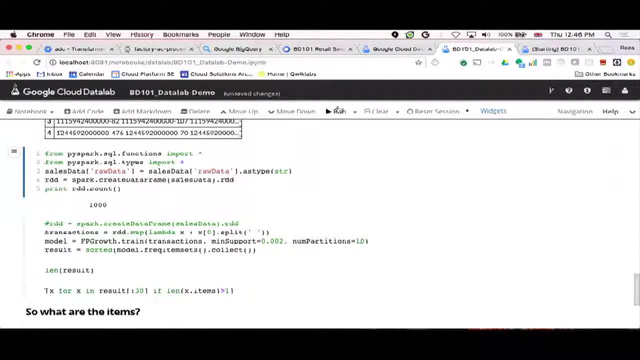 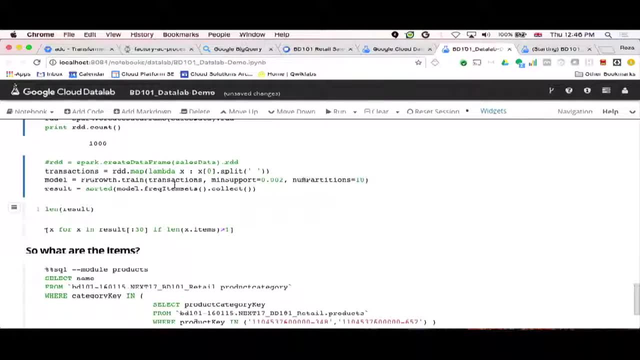 I'm going to get this put into an RDD. Those are the 1,000 data sets that are there. Next step, I'm going to run the algorithm, which is this: FB grow from Spark. Look at the results. It gave me 36 results. 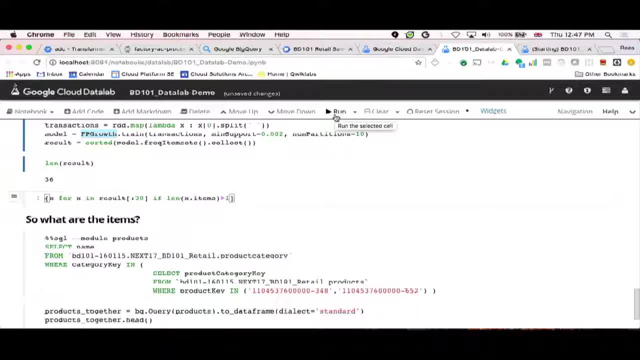 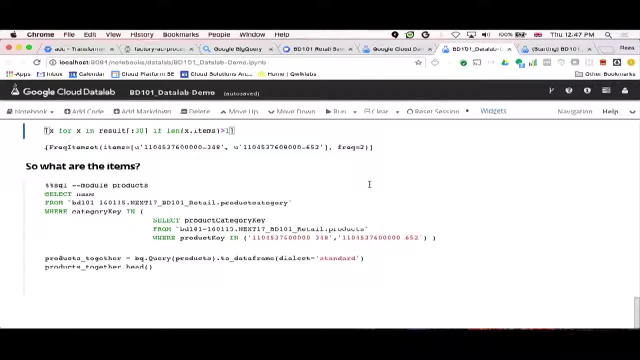 I'm going to look at where item is bigger than 2.. I'm going to the details of that. So, as I mentioned before, BigQuery does cache results. This morning I had run the limit 1,000, so I don't have to do some typing here. 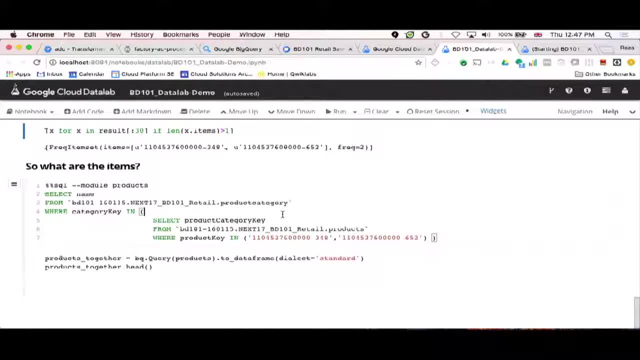 So the first thing I would do after getting some results back is go and check them. So what I'm doing here is I'm going to use those product IDs, go back to my data set and see what is it that people buy together based off category. 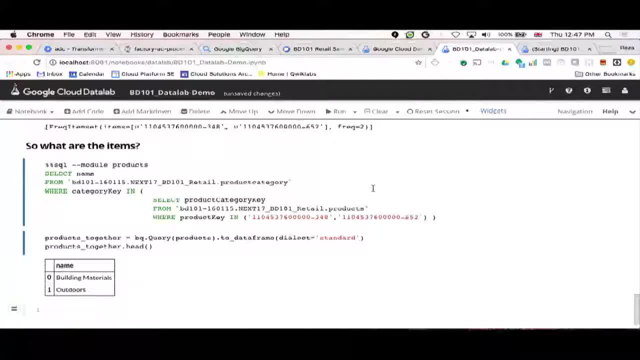 So this seems building materials and outdoors, OK, interesting. At this point we now have most of everything that's ready to pass to a data engineer. They can then go and productionize this and churn out the information across the whole data set to start figuring out what are. 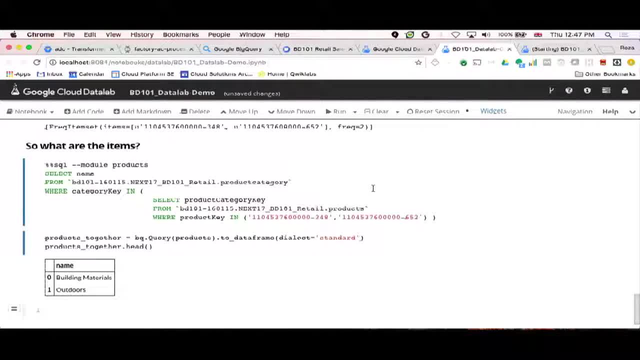 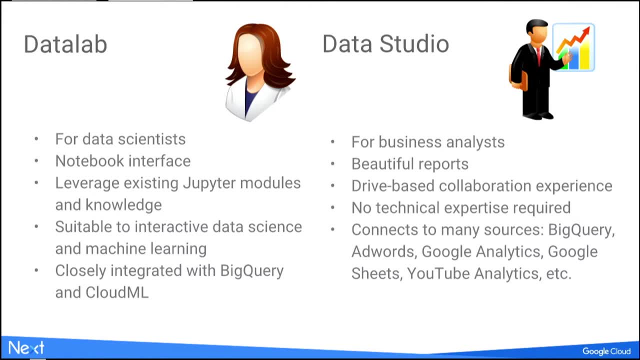 the items we should recommend on our website. OK, PHILIPPE RIGOLLET- Back to the slides, please. Thank you, Reza. And so this was Data Lab for our scientists. Since this is an intro session, I don't. 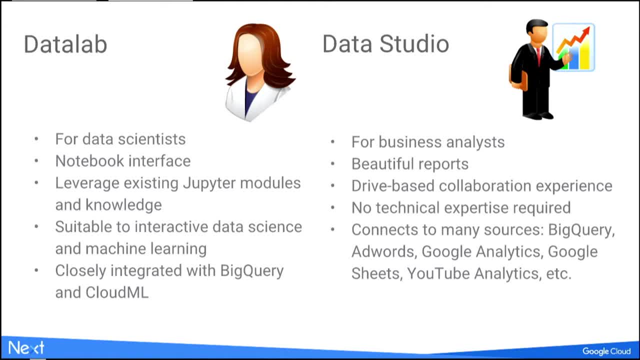 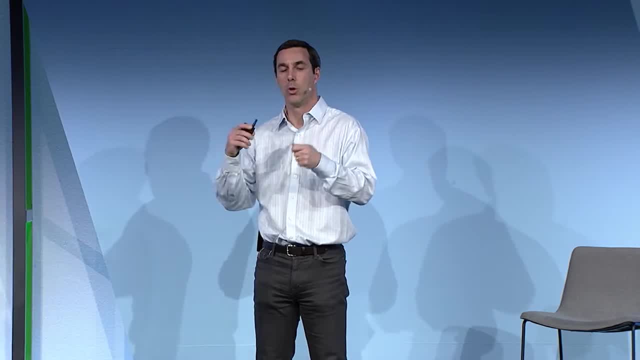 expect. many people in this room are data scientists, But people in your organizations or people you might work with who have that skill, that is the tool that will be most familiar with them and allow them to collaborate with you on the same data in Google using the tools they want. 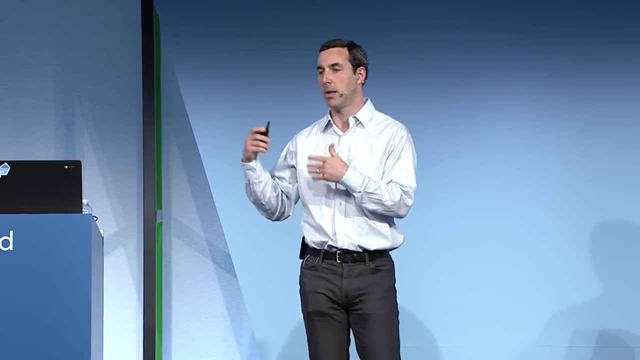 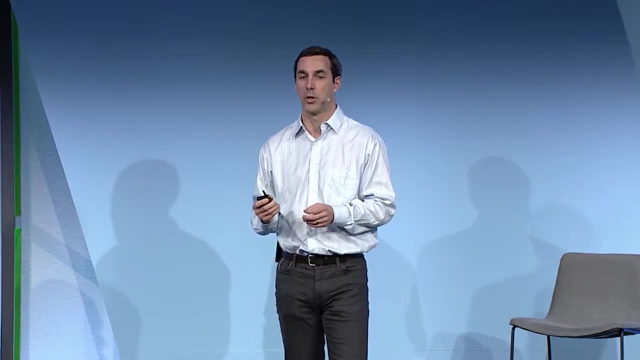 For more business analyst type of people, people line of business managers, people who are more on that side of the business. one tool that's on the platform that's quite useful is Data Studio for reports, And that's another serverless tool in the sense. 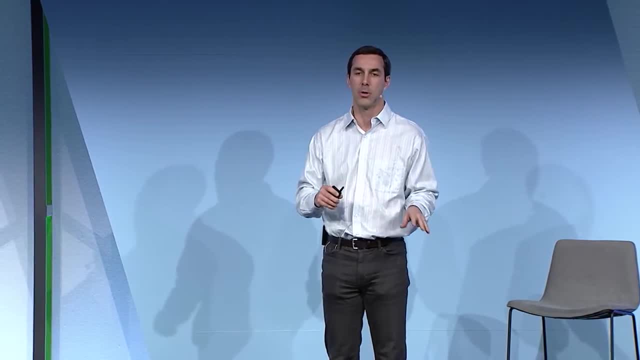 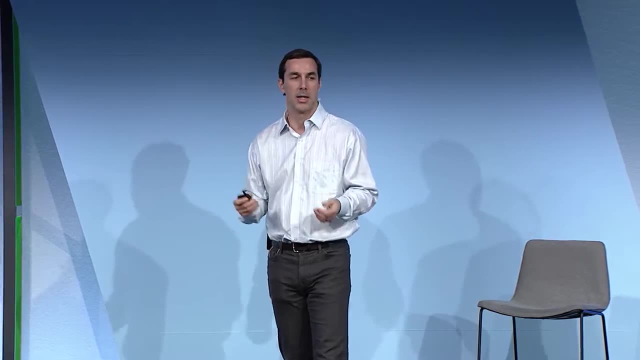 that you don't install anything either on the client or on the server. It works like Google Drive. It is a collaborative environment And so I expect many of you are familiar with Google Drive, and having a presentation and documents and spreadsheets And Data Studio allows you. 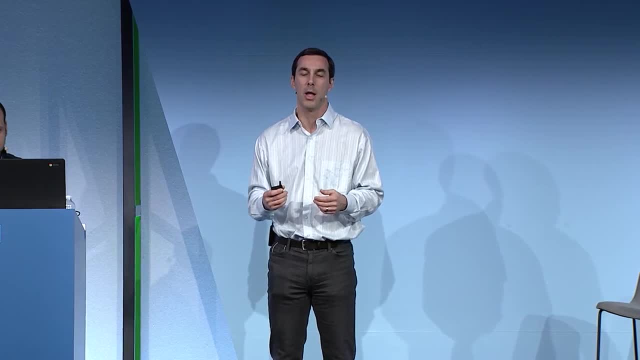 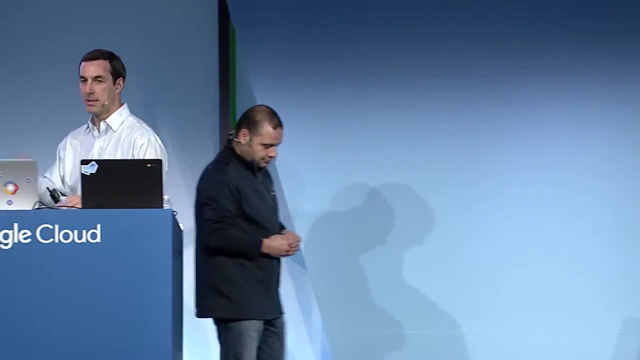 PHILIPPE RIGOLLET- Thank you. And Data Studio allows you to use that exact same collaboration model for creating and sharing beautiful reports on the platform directly. And so let's look at it in practice. if we can switch back to the laptop demo. 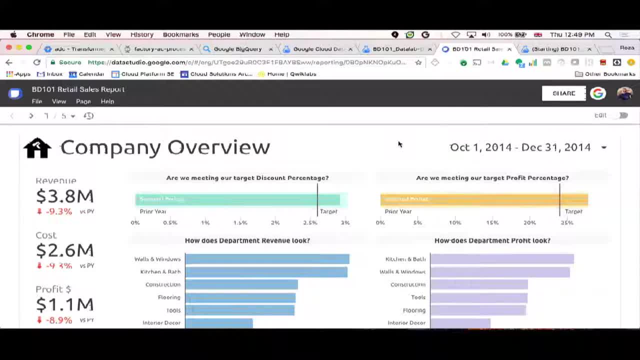 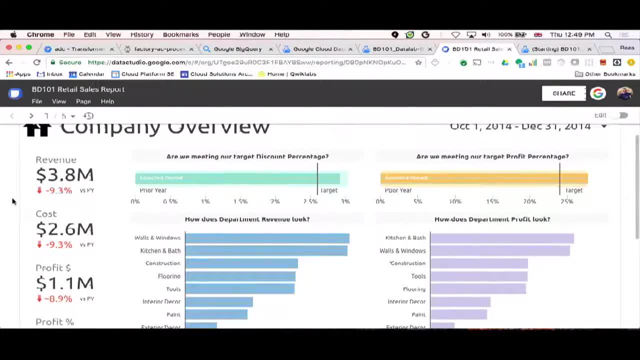 So do you have it? Yeah, So this is an example of a report dashboard in Data Lab which has some calculated value on the left side. So remember, I mentioned in the data prep demo once I've extracted the time of the ad and the time of the transaction. 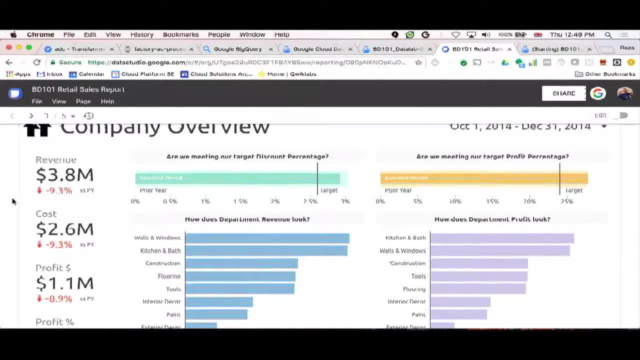 I could do the calculation back then in data prep, Or I could leave those two values nice and clean and then do the calculation in Data Studio and as part of the creation of this report. Either way would work. I can look at my various metrics here compared to target. 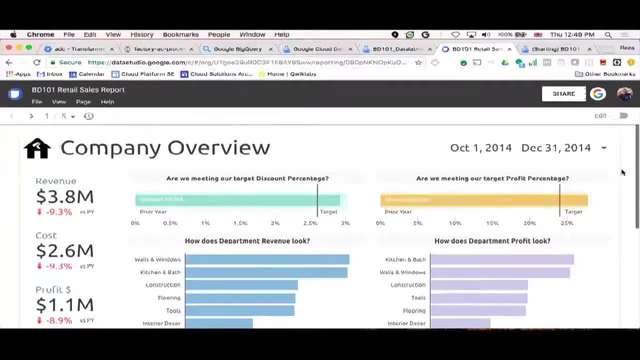 et cetera. There is the all of those array of data that I have here, And I can see that I have a lot of data here, And I can see that I have a lot of data here, And I can see that I have a lot of data here. 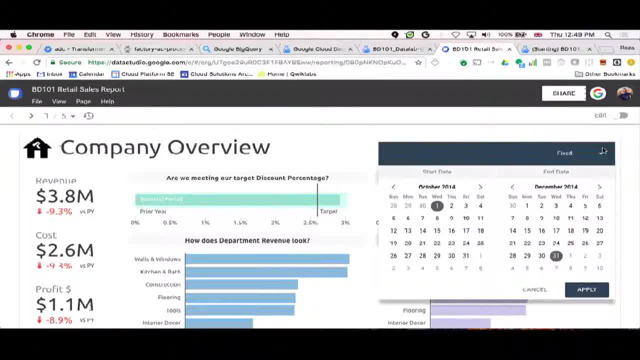 All of those areas are being controlled by that data item here which was put there. So, instead of looking at the last quarter of 2014, I can go back and look at the full year, And so here I'm acting as a viewer of the report. 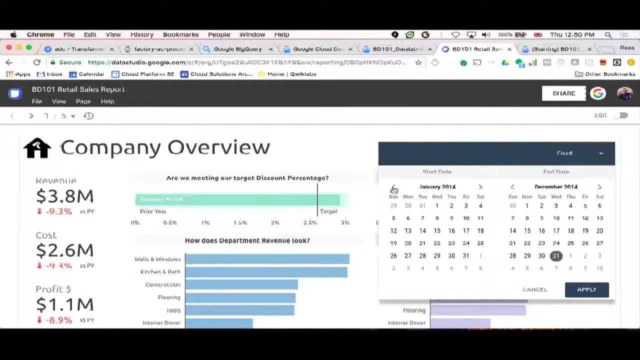 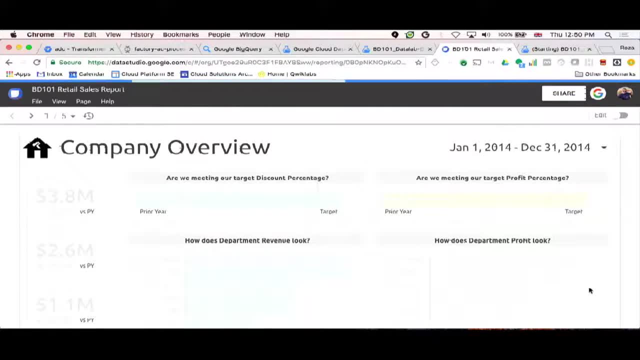 not as the creator, And so anybody with whom you've shared the report would be able to do that and adjust the report to get to what they're trying to get to. So we just apply. It gets recalculated such that the revenue is now. 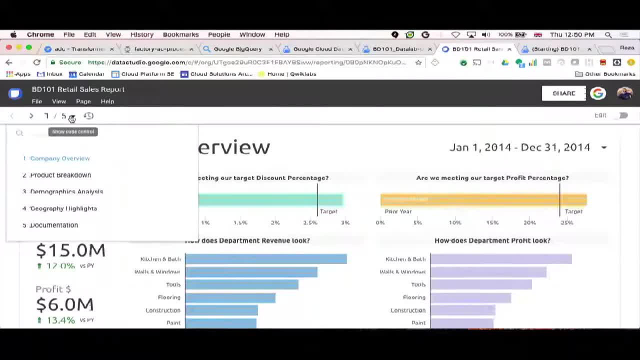 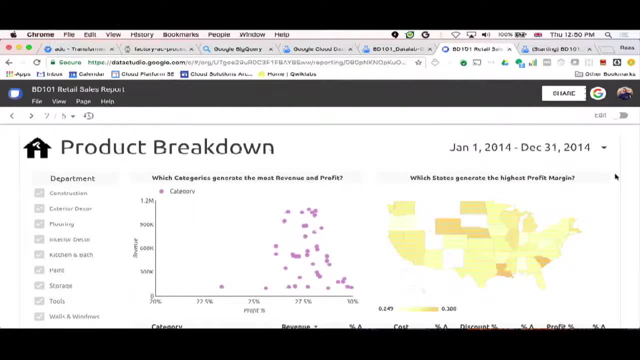 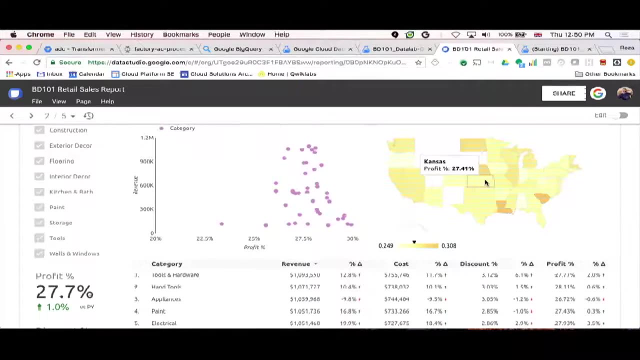 the full year revenue, et cetera, And so that's one page of the dashboard, And there are other pages that shows other kinds of views, like, for example, here having this geographical view. So this one represents the profit margin for various stats. 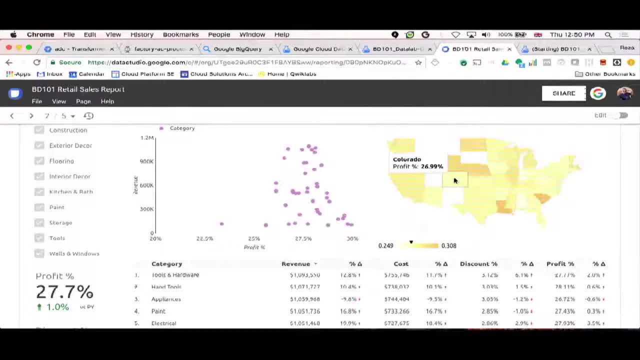 Can hover over the various stats And automatically it recognizes in the data geographical information and offers visualization specifically for that. allow you very easy, as a non-expert, to put together. dashboards. can look at the product, so the demographics, so you'll find out. 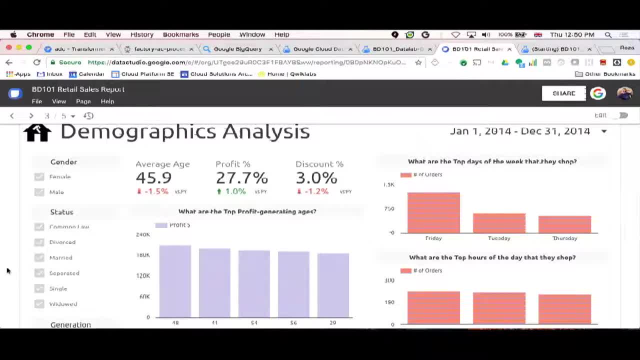 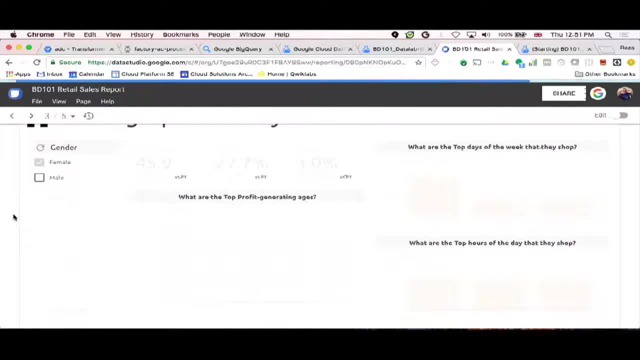 more about the users and what you know, other data based on the customer tables in that retail data set. do some filtering on that so you know, remove the male users, for example, to filter down to know, just to just, let's say, just all the female except the baby boomers to you know, and then you can drill in and 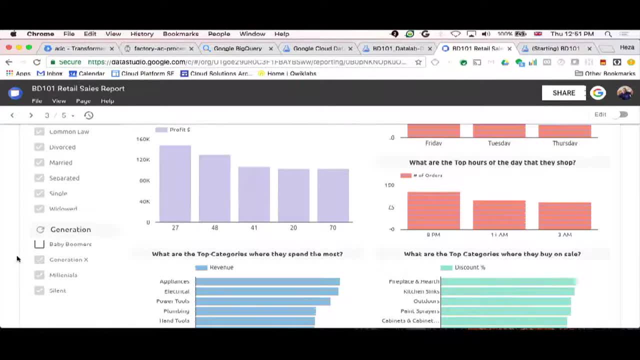 automatically those selectors, whether the dead selector and or those population characteristics selectors in this, in the case of this dashboard, where we're configured to apply to all of the visualization on this page. so that's the experience as a user. somebody, someone has shared that with me. I know nothing. 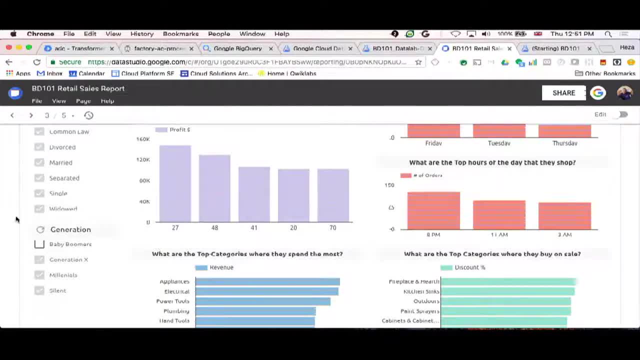 about BigQuery or anything. I just have that easy dashboard that I can interact with and and get inside for myself. now let's look at how that dashboard actually gets created and, Reza, if you want to, yeah, sure that in action. so if, okay, what I'm gonna do now is do a little bit of 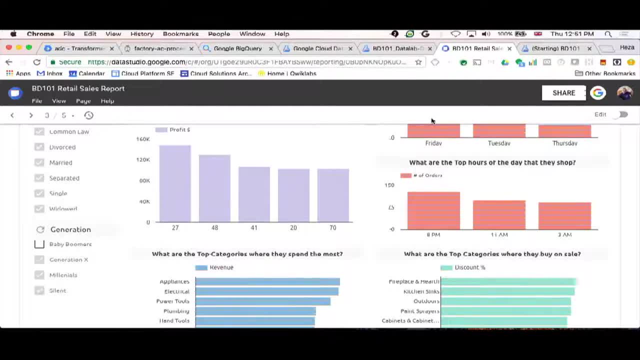 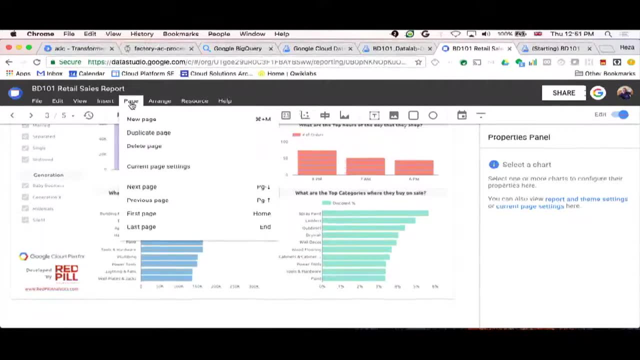 UI, and there's a good reason. they usually don't let me near any UIs, as will soon become apparent. so I'm gonna first of all put this in edit mode and actually create a page. so create new page. so at this point I have a blank. 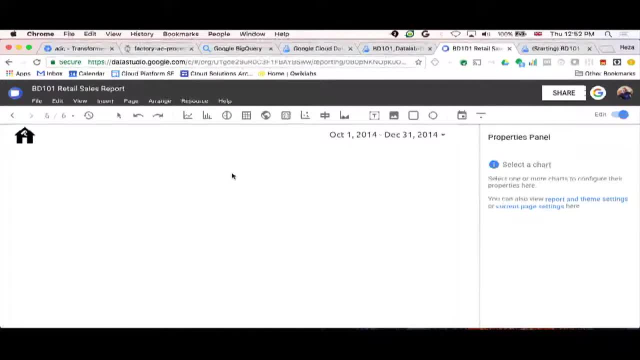 page to start building out some components on, and what I'm going to do is build out one of those first graphs that we had in that first page. so what I want to do is a bar chart. I'm gonna put the bar chart down and it's. 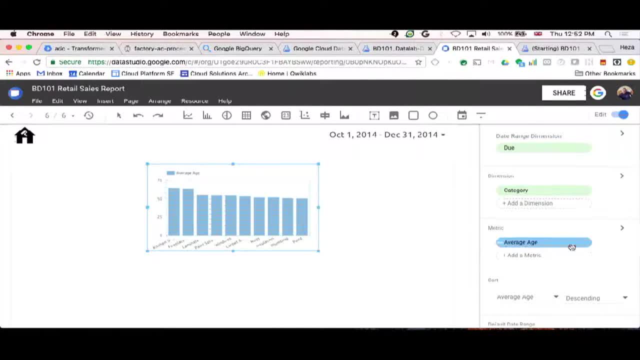 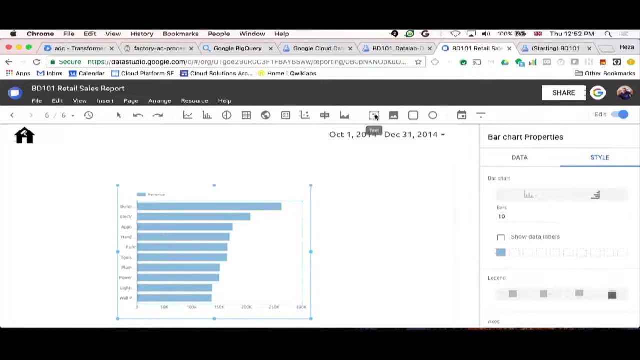 already given me some options. it's actually chosen. average age is a metric. we want the revenue okay. revenue selected okay. if I recollect the, the style of the graph on that first page was horizontal, so let's turn that horizontal. there was also a text bar at the top. let's just add that. and my chart. it was also gray and black line. 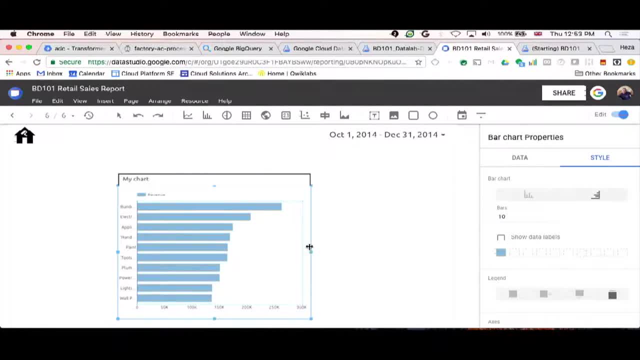 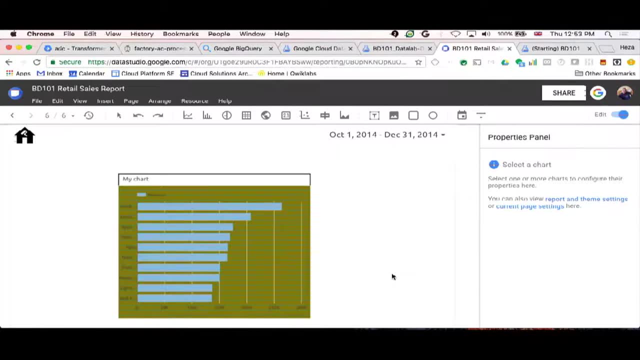 let's put a weight around it, okay, and as I have very little UX skills, let's pick a color that I think is very beautiful, gorgeous, that looks beautiful. so I think I might need some help from someone with a little bit more UX skills. so, William, perhaps you could come and 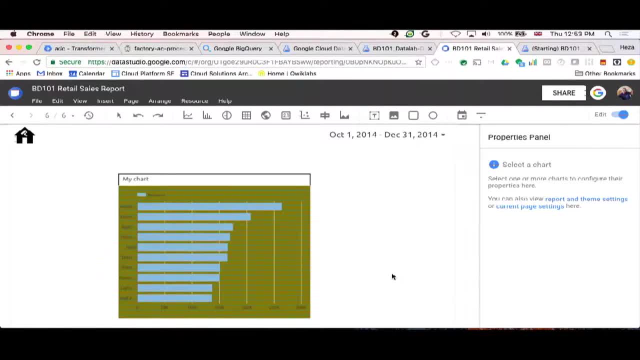 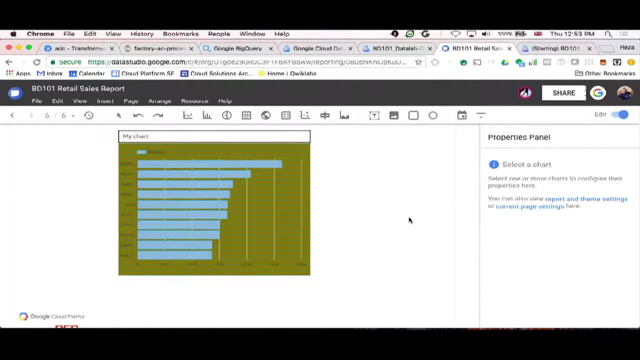 join me in this. so since that was shared, you know, using the, the usual model now I get, so you see my icon here showing up because I joined that dashboard and I can beautiful picture. that's me and I can go and try and rescue this chart from Reza's hand. so that's before people start leaving the room, let me try to. 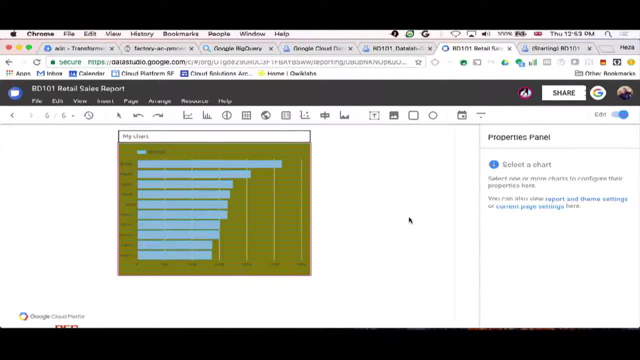 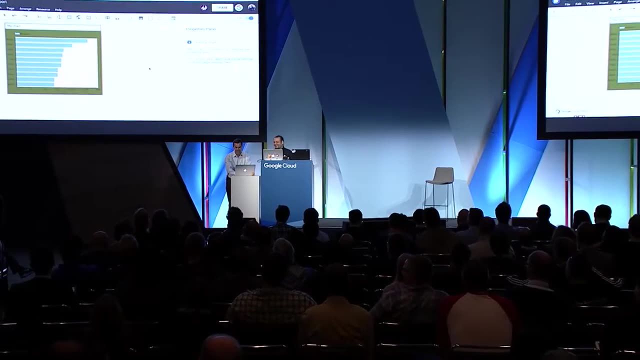 change the color here, and this is my look- no hands moment, and so go to the style. so basically, what I'm seeing is the same thing Reza was seeing when he was doing the edit himself earlier, and so chart background, let's make it like a nicer pink. that was that better. it's less, less aggressive, and then I like 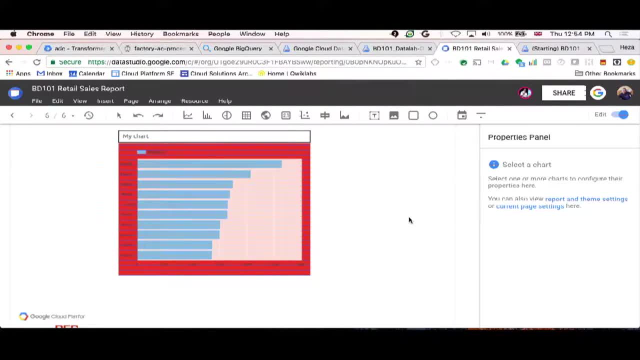 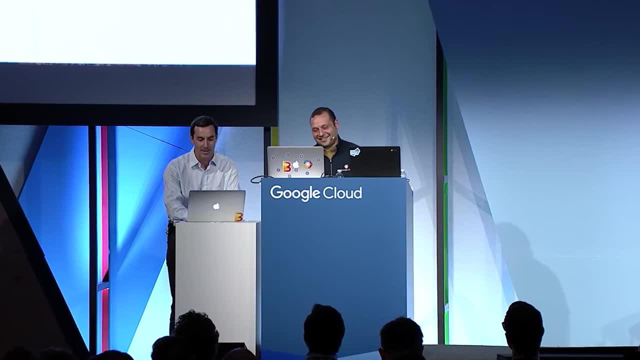 this. okay, now you can't read the day job, right? anyway, hopefully you guys will not. we haven't ruined your appetite. for the rest, I'm let's do something maybe more useful. I'm gonna add another chart, and so well, speaking of appetite, let's do a pie. 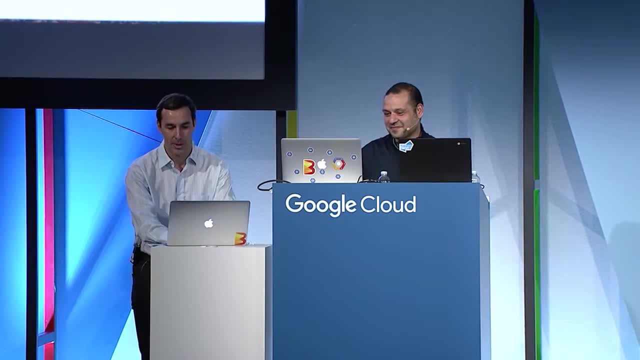 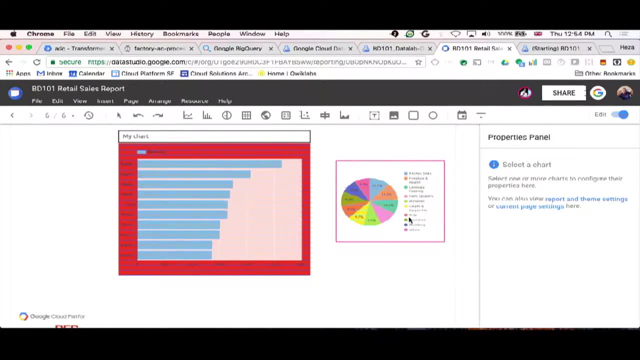 chart there. it is showing up here, and so you know by default. the data was the product categories. here I'll make it bigger. so, Reza, you put yours right in the middle. you don't give me any room- and so you know by default. here we had. 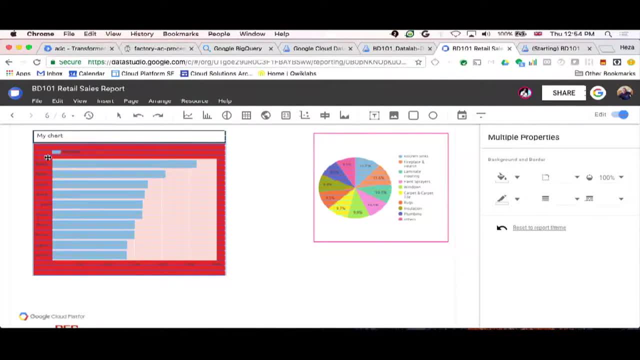 the product category. oh, thank you, then I can expand mine. and then I know, instead of that I can put other dimension, like no, the page of my users or the gender of the user. so you know, just as I composed, the key thing here is, for those of you familiar with Drive, collaboration that's. 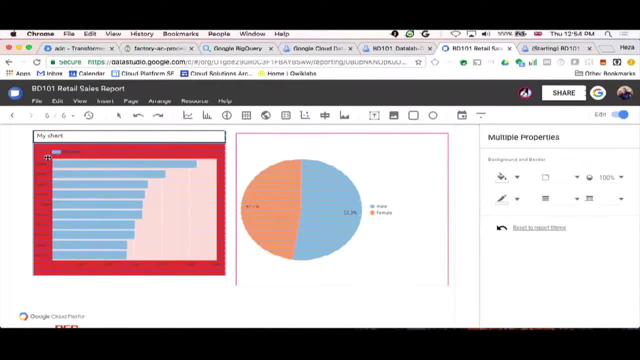 the usual experience where you see the other person and you can together collaborate, and so let's see like- let's assume, we reach perfection. this is both beautiful and useful. please show us how to share it. 50% correct, so we're gonna share this document. if you use Google Drive, this will be very familiar with. 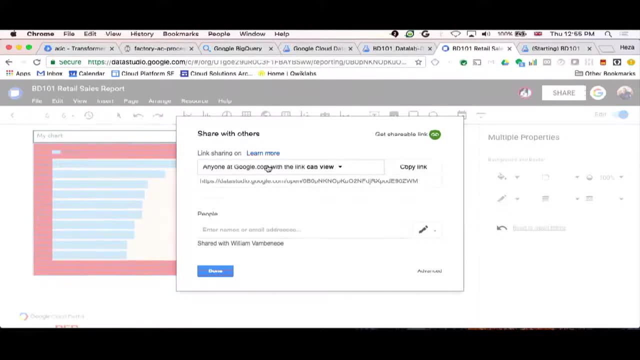 you, and so it's already shared. that list link is already shared with my domain, my company, googlecom, So anyone with that link can access this data set. If I wanted to restrict it further down, I could choose emails to limit who has access. 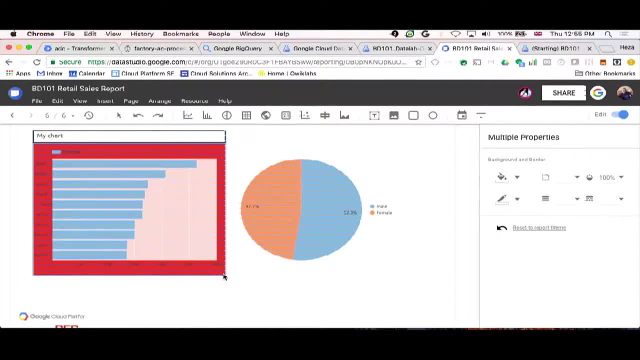 to this particular data set. OK, so back to William WILLIAM BONVILLIANI- Thank you, Reza. So yeah, that's the typical Google Drive sharing model, so very useful collaboration. If you can go back to the slides, please. 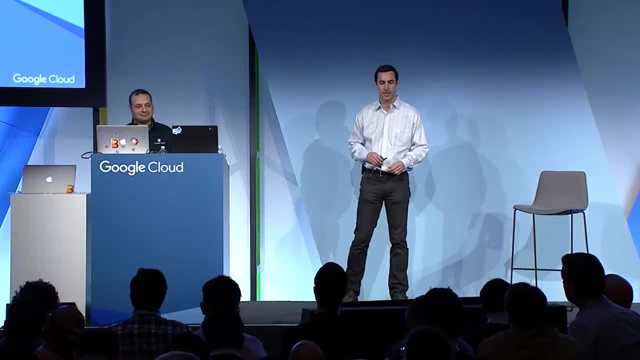 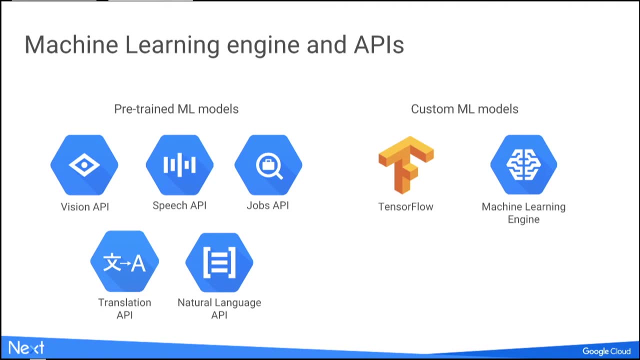 WILLIAM BONVILLIANI- Thank you. And then another aspect here that we want to finish on is as far as big data processing more and more, that also includes machine learning, And so we announced yesterday that Machine Learning Engine. 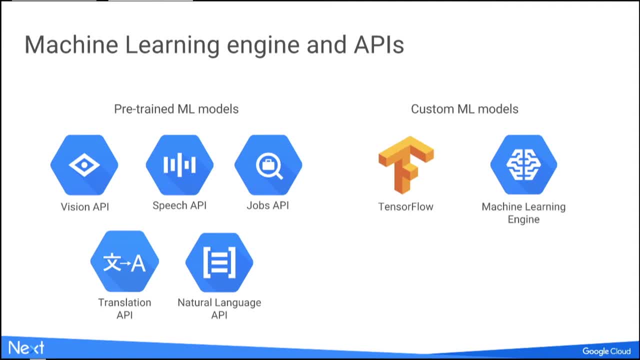 is now GA. That's out of scope for this session. Plenty of machine learning sessions here. One set of APIs which are actually relevant to people who don't have to be machine learning experts is the fact That you can use APIs that expose models. 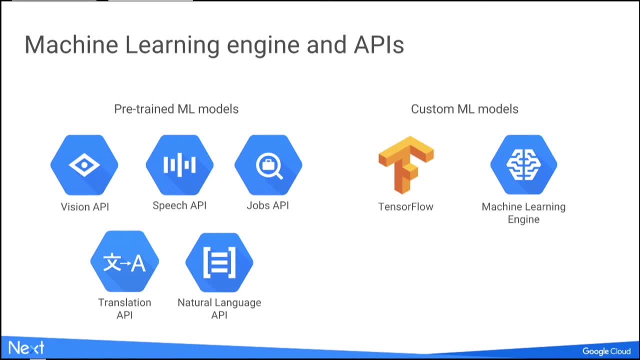 that Google itself has trained using our own data. And so there's the Vision API to extract insight from images: what's in the image, recognize location, landmark and a lot of things like that Speech API to automatically transcribe voice into text. 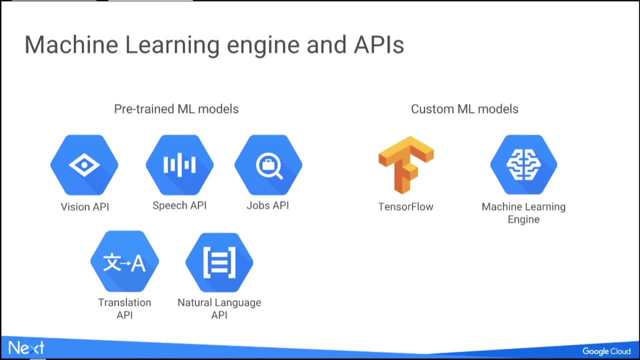 Jobs API. that's a pretty specialized API, But I think that that's where the industry is going In this case: having an API specifically for matching candidates resumes to job opportunity And something that goes way beyond typical keyword matching and really has been trained on really, really large amounts. 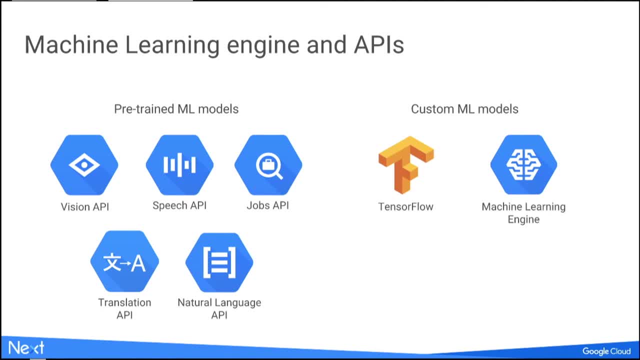 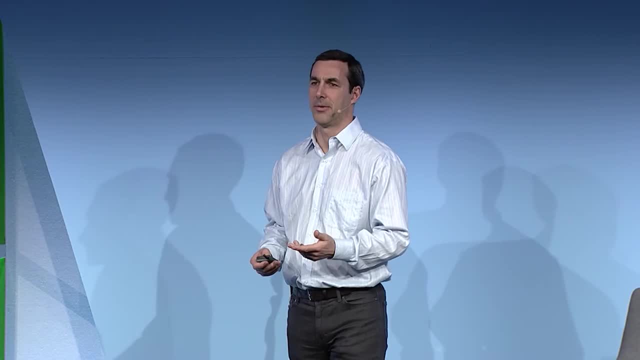 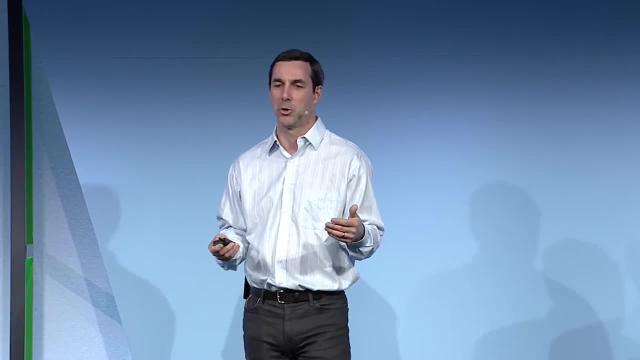 of data and has much more insight about what actually makes sense for matching. Recently I was looking for somebody who passed me a candidate who has Apache experience- And I mean Apache's foundation- And he actually had worked on Apache helicopters. Thank you, 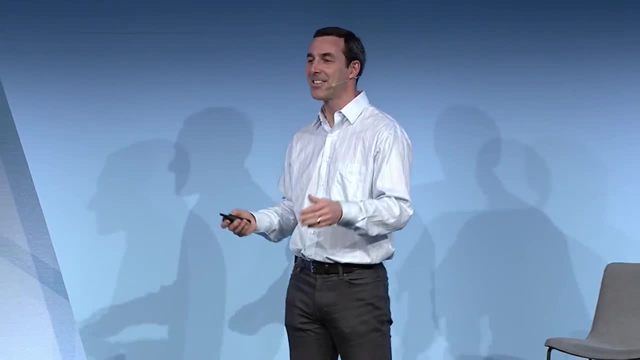 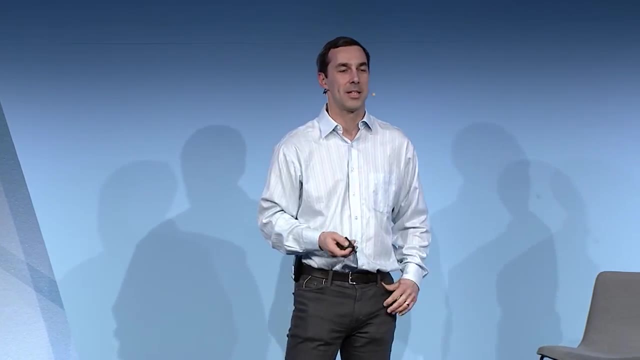 That's not exactly what I was looking at, So that's the kind of thing that they know You can go beyond keyword matching and people who are quite relevant for what you're doing. Another one is Translation API. I'm sure many of you have used it as consumers. 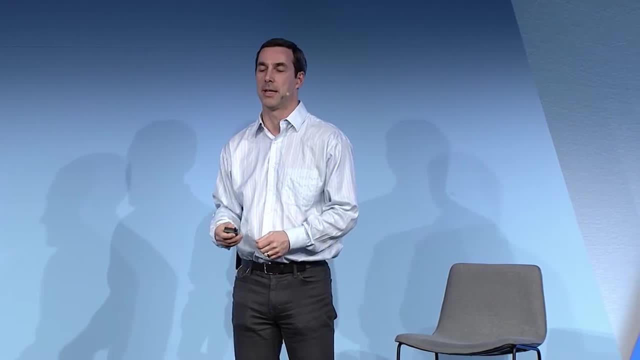 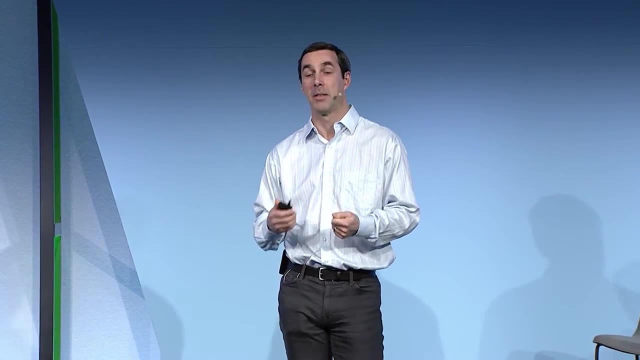 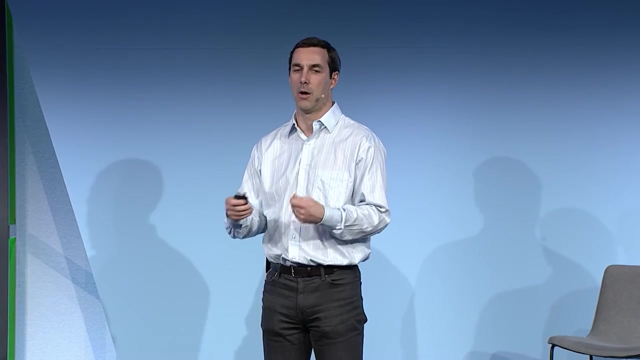 It's available as an API to use in your products and in your data processing pipeline. And finally, the Natural Language API, which takes text and tells you what the text is talking about. You know which people, which location, what's the tone of the conversation? 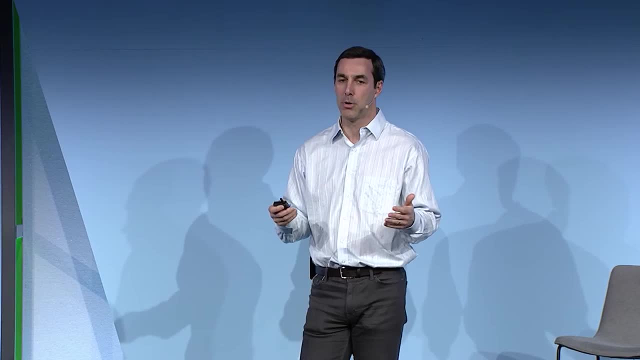 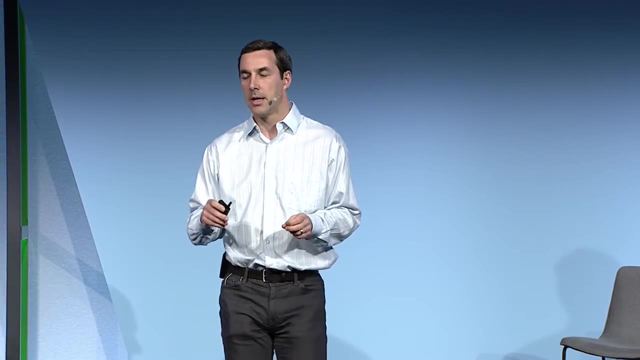 Are people happy, unhappy, and things like that. So that's an example of something that anyone, not a machine learning expert, can start using, And so, in conclusion, I think what we try to do here is to do a mix of explaining the value of serverless processing. 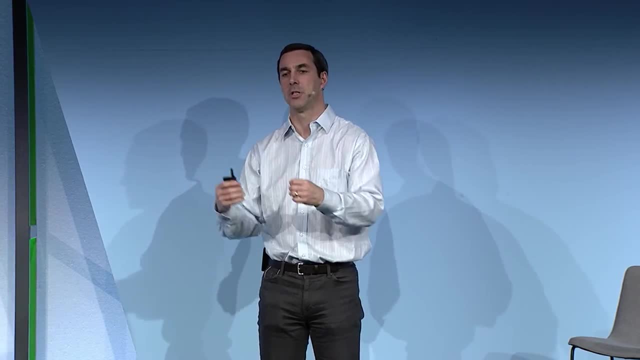 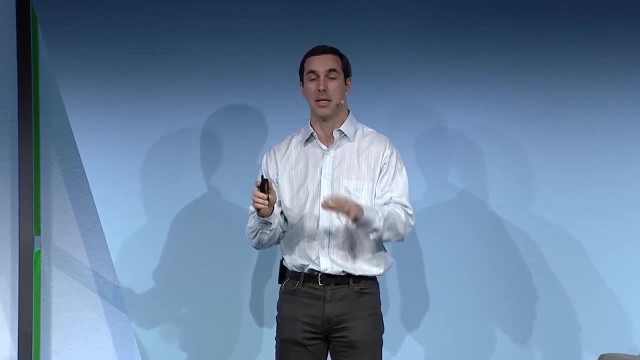 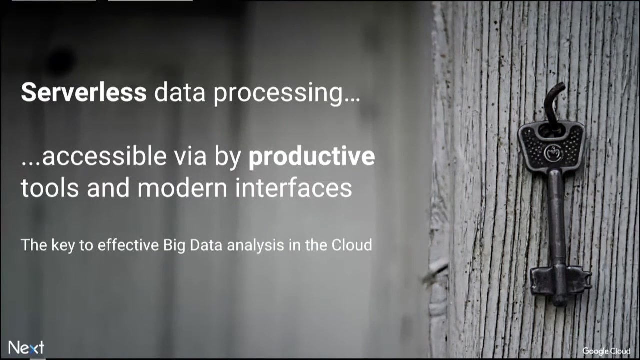 and how it brings scale, speed, efficiency and cost efficiency to data processing, but show how the way to use that in many cases is a very easy tool, And so we did a demo of Data Prep for data preparation. We did a demo of data lab for data science.